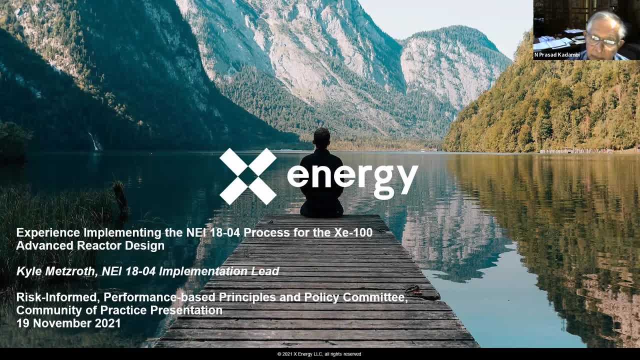 center for RIPB, with all the collection of community of practice sessions that we have in place. You can find more information on RIPB on the RP3C web page of the ANS website. RP3C initiated these community of practice webinars on RIPB to enable 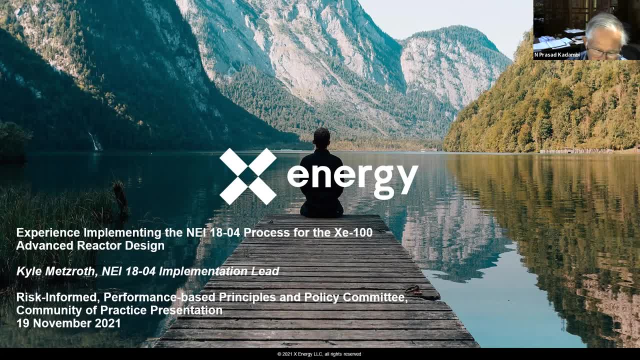 practitioners of RIPB approaches to share their knowledge and experience. We have generally scheduled these on the last Friday of every month. This month is an exception because the last Friday of every month is the last Friday of every month. Friday falls on Thanksgiving weekend. I'm very appreciative that Kyle Metzroth of representing 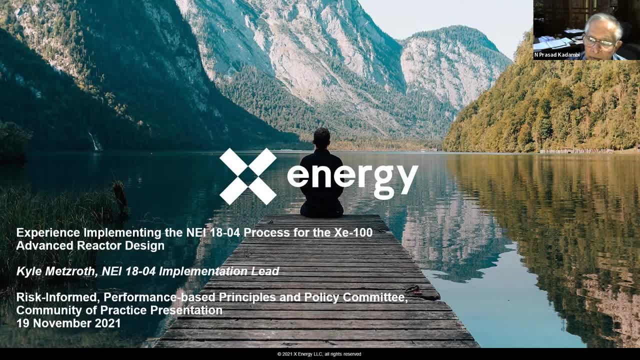 X Energy has agreed to speak about the experience and knowledge that X Energy has developed as a result of using RIPB methods, And he will talk about this in the context of the NEI 1804 document that NRC has actually endorsed in a regulatory guide. So Kyle the floor. 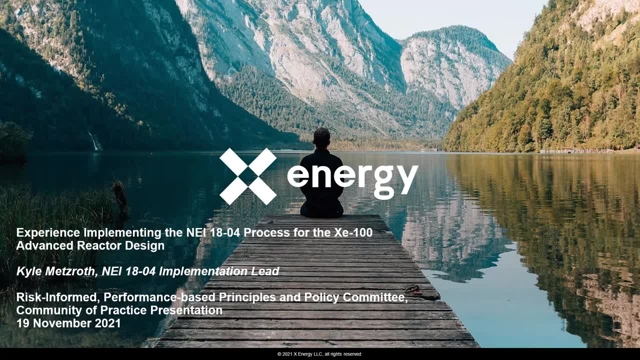 is yours, Kyle Metzroth. Thank you, Prasad. Just to confirm. can you hear me, okay, Prasad Sinha? Yes, I can hear you, Kyle Metzroth, Perfect, Thanks. Well, thanks everybody for joining today and to this talk. My name is Kyle Metzroth. I work for NPR Associates. 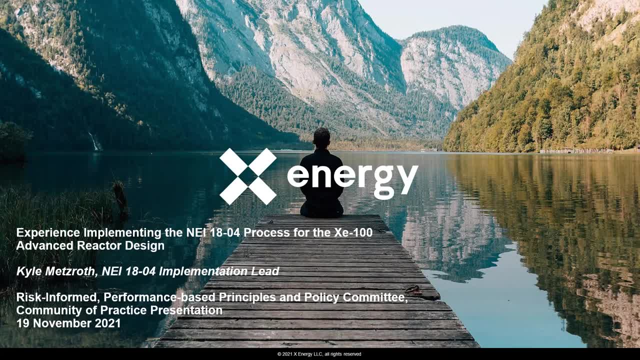 but I've been working with X Energy over the past year, supporting them as their implementation lead for the NEI 1804 process, And so what I'm going to be talking about today is a little bit about the experience that we've had in implementing the process and some lessons. 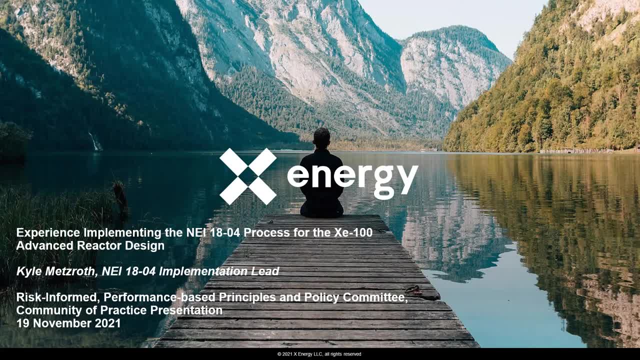 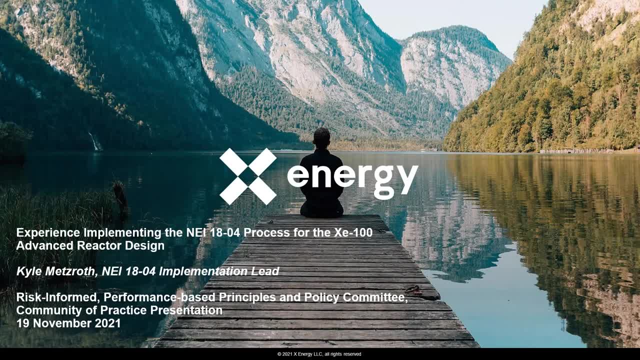 to start with the process. So I'm going to start with the process. So, again, that's my role actually is. I would say I play an integrating or interfacing role between the various groups within X Energy, trying to bridge the design, organization, safety. 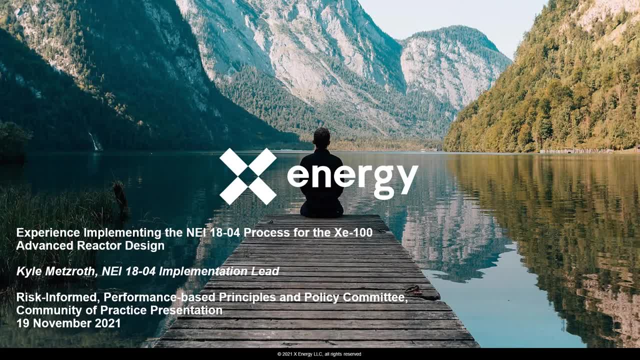 analysis, PRA and licensing organizations And driving the implementation of the process, making sure all those groups are conversing with one another, all the insights are shared, etc. So that'll get into it My background, just for those. I'm. Kyle Metzroth Supervisor career問: Prasad Sinha, I've been working with эта Shell in about six years or so or since that began, Like I understand. but how many people have worked with願 dpnS tyrk around these? 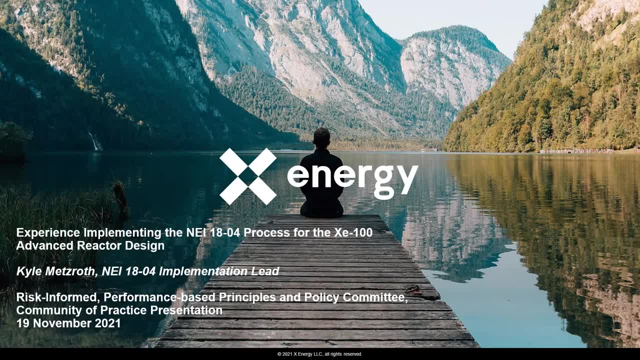 new to this particular community, So I have some PRA backgrounds. My PhD dissertation was actually in dynamic PRA methods. I haven't practiced PRA methods much since that time. I've done mostly safety analysis work, some for the US Navy. I worked in the design of the Columbia-class and 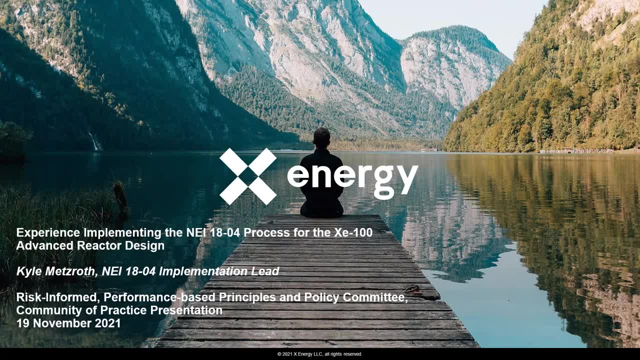 Virginia-class submarines And since my time at NPR I've done mostly nuclear safety work. So I would say in all of the various elements of NEI 1804, I wouldn't call myself an expert- in each individual one- We have a team of experts that help to implement the various pieces. but 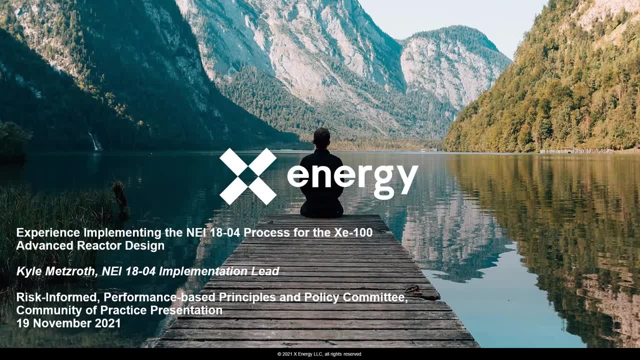 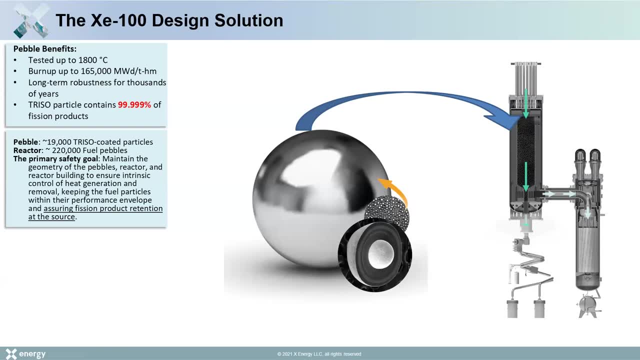 sufficiently dangerous in each, I suppose. So to give a little bit of background on the XC-100 design itself for those who may not be aware. So the XC-100 is a pebble bed modular reactor design utilizing triso fuel. So a depiction of the 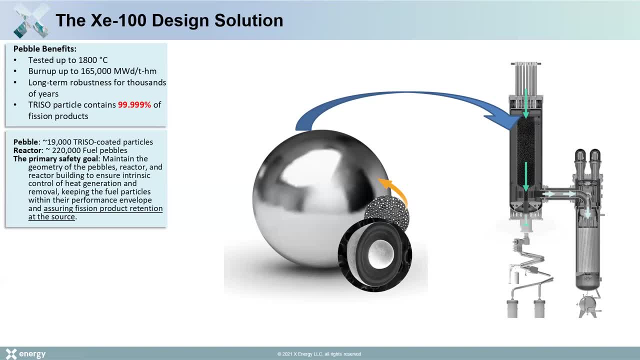 design of the XC-100. And its current concept is here on the right-hand side. So we have the pebble bed core, where pebbles flow in from the top down through the bottom, through a fuel handling system and then are. 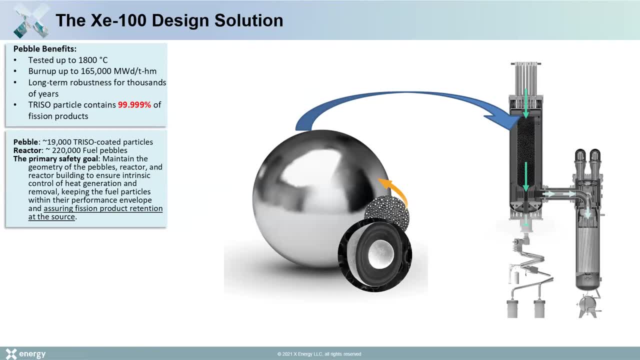 recycled back up to the top. The core is downflow. So helium enters the core from the steam generator up along the graphite reflector over in this direction and then turns down. The flow goes down through and then over through a cross vessel and then into a helical coil steam generator. 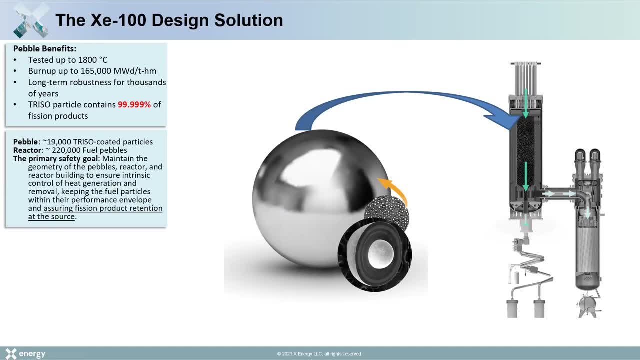 There are two with two helical coils, Helium circulators driving the motion of helium through the core. The safety case for the XC-100 is similar to that for many other past HTGR designs. The main safety case lies with the fuel and maintaining temperatures less than the point. 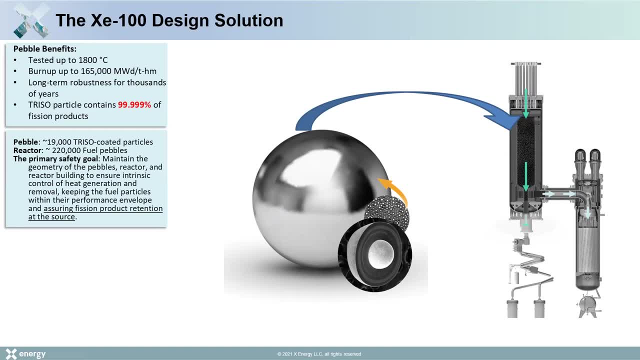 where the fuel begins to see issues. So the XC-100 design utilizes the UCO triso design. The fuel has been tested up to 1800 C, very high, very good performance. up into those temperatures And you know so. the reactor has the ability to remove, you know, all of its decay, heat away. 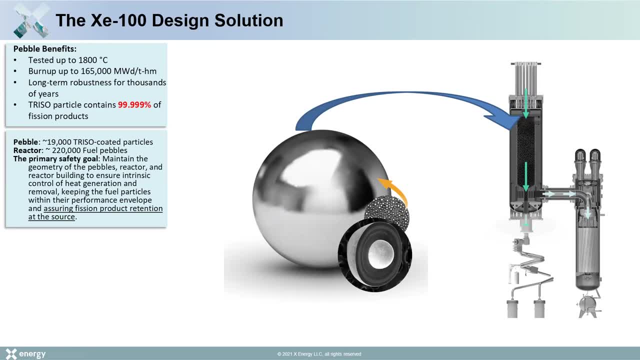 passively right, So no active cooling systems are required. And so, again, the majority of the safety case rely, you know, rests in the fuel, the ability to conduct the ground and the inherent safety of the plant itself. And so, you know, given these inherent safety features, you know, 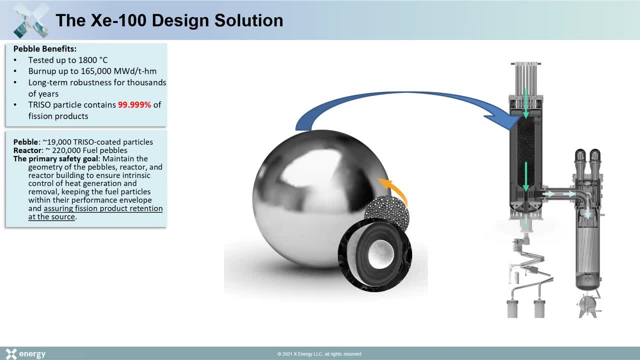 the X-Energy team, you know, is strongly leveraging risk enforcement and safety features to ensure that fuel is in good condition, performance-based methods to be able to take advantages of that inherent safety. You know we don't need a substantial amount of active systems to be able to perform during. 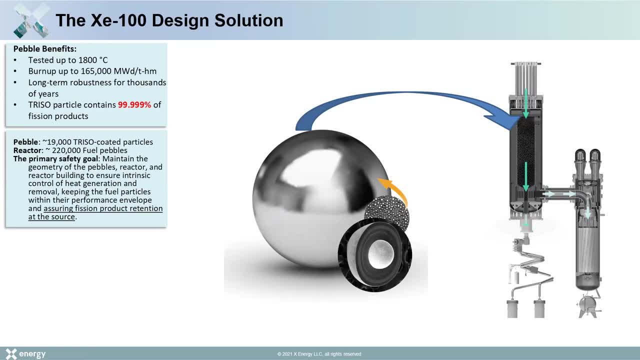 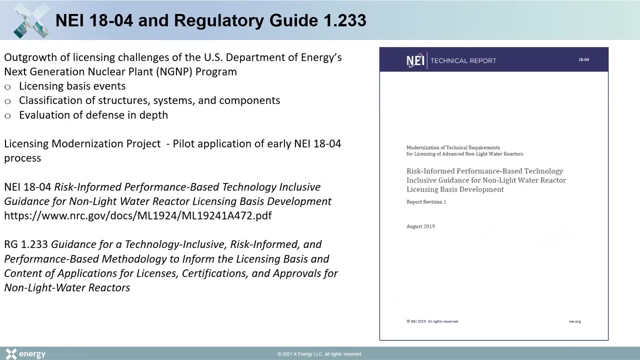 any design basis, accident scenarios And so really leveraging that inherent safety, you know, to have a cost-effective design. So NEI 1804.. So X-Energy is committed to utilizing the NEI 1804 process. You know it's a risk-informed, performance-based process, really focused on non-lightwater. 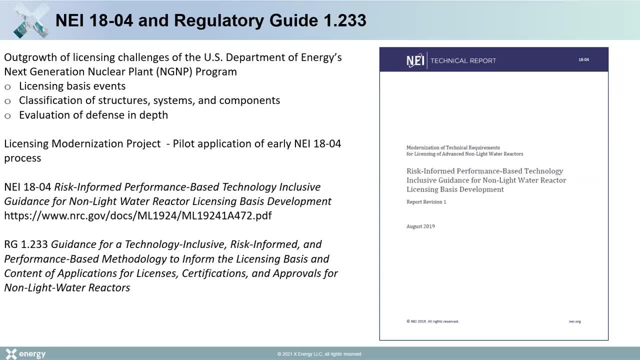 advanced reactors, You know, and the key aspects of the process are that it helps with selecting, licensing, basis events, classifying structures, systems and components, and also has a holistic evaluation of defense in depth, As many people are probably aware- and I don't know the full background of everyone on this- 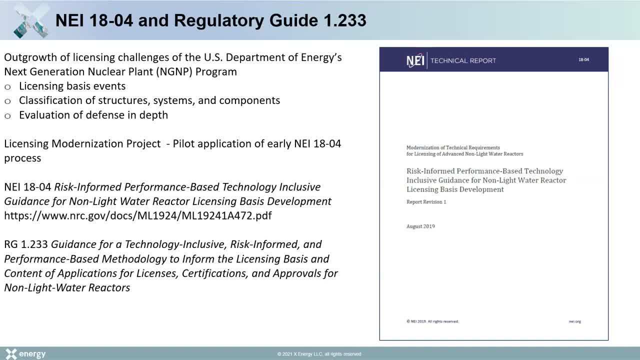 call. So I will be going into some explanatory details about the NEI 1804 process, just to make sure everyone's on the same page. But I don't consider this an NEI 1804 tutorial, just enough to at least provide context to. 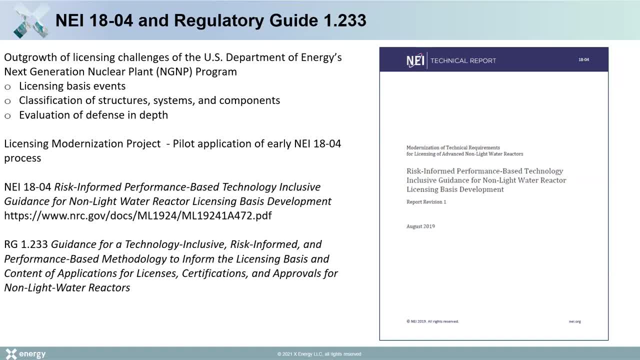 the things that we're doing. So, as many people are probably aware, you know, with existing, the existing lightwater fleet, a lot of the- you know- accident cases that we look at design bases have been built up over the course of years of experience. 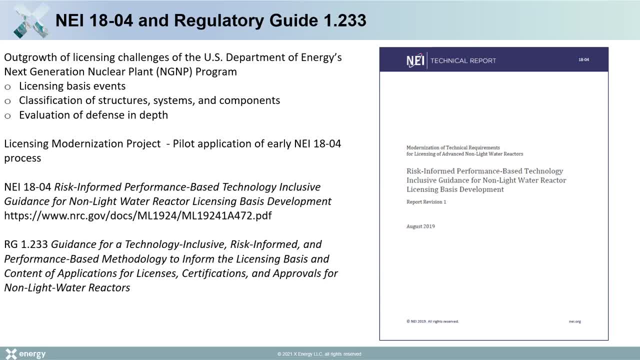 And you know we don't necessarily have all that for advanced reactors And nor do we want to live to the same standards. So you know the 1804 process allows you to leverage the PRA to be able to build those. 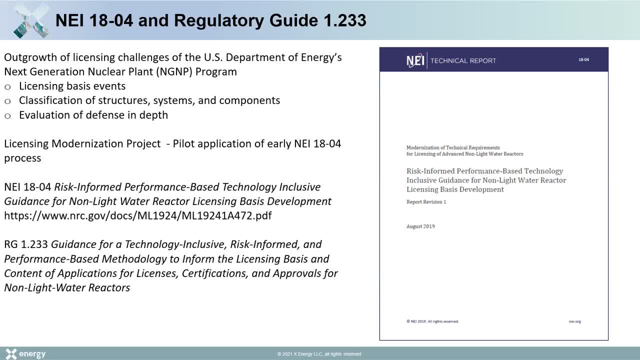 licensing events and leverage the importance of various SSCs to risk and nuclear safety to be able to classify the structure, systems and components you know. accordingly, And using an early version of this process that we'll be going through today, you know, 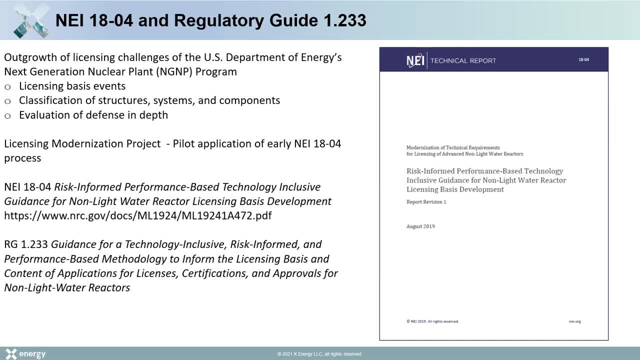 X-Energy has taken a part in what's known as the Licensing Modernization Project- which I think probably many people on the call are aware of- where there were several advanced reactor companies that went through an early stage of the process to demonstrate its capabilities. 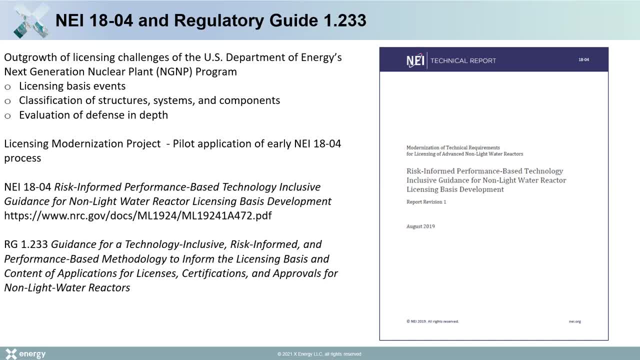 And, as a matter of fact, a lot of what I'll be talking about today is going to use that as an example. We've gone much farther than that since then, but just since this information is currently publicly available, I'll be using it as sort of a backdrop for the conversation. 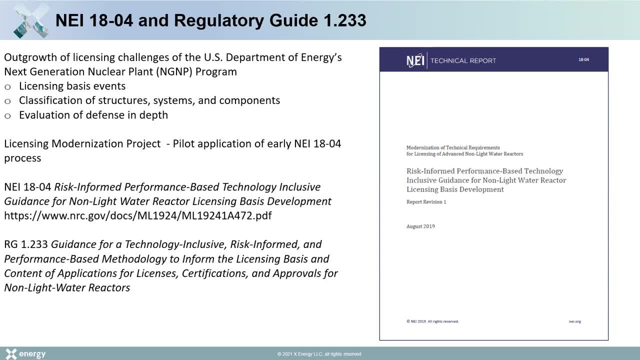 So X-Energy participated in this pilot. We actually leveraged a lot of the information. There was a lot of information that was gained from it to help inform the design and I'll be discussing that a little bit. For those who may not be aware, this is, you know, a link, a reference to the NEI 1804. 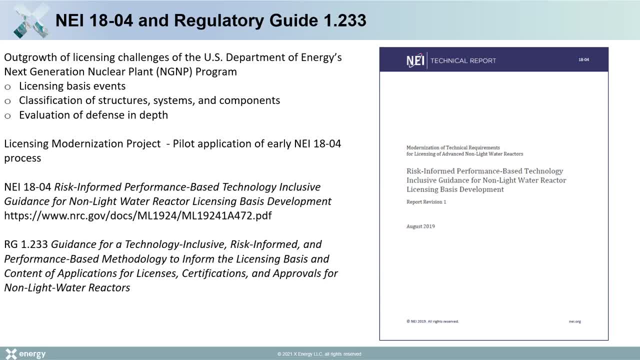 document And you know, as Prasad mentioned at the beginning of the discussion, that the NRC has endorsed NEI 1804 as a risk-informed method for forming the licensing basis of advanced reactors. you know, with some clarifications. 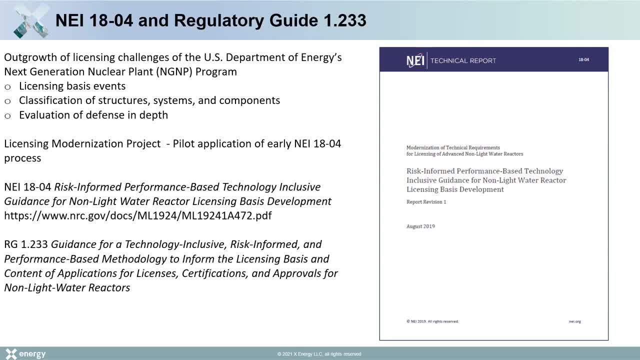 But you know, largely I've adopted the guidance in the document And, as I mentioned, you know we're committed to following this approach because we see it as a way to maintain high levels of inherent safety but at the same time balancing cost. 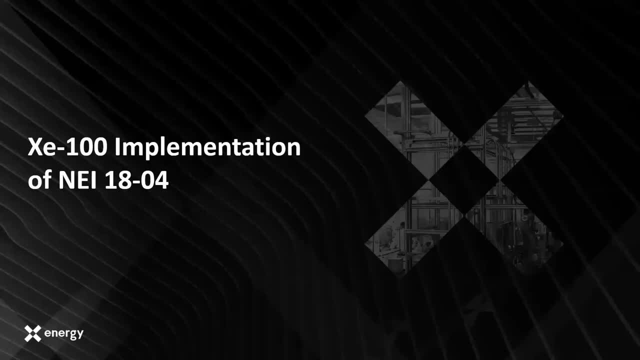 as well. So I want to get into now a little bit of how we've implemented NEI 1804.. You know, so I'm limited to some degree on things that we can talk about at the time, just because of proprietary information. 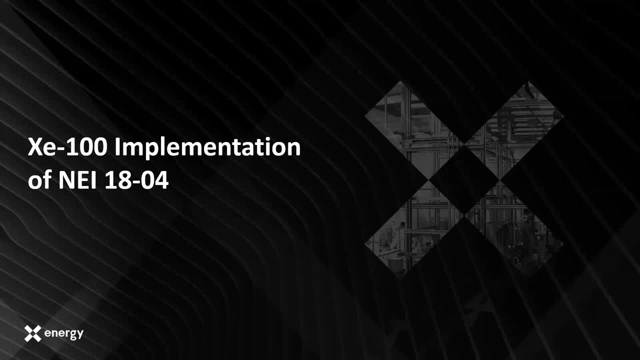 But what I'm going to try to do is, as I mentioned before, we're going to use the licensing modernization program, which I'll refer to as LMP, LMP pilot. that was performed as sort of the backdrop to talk about it. 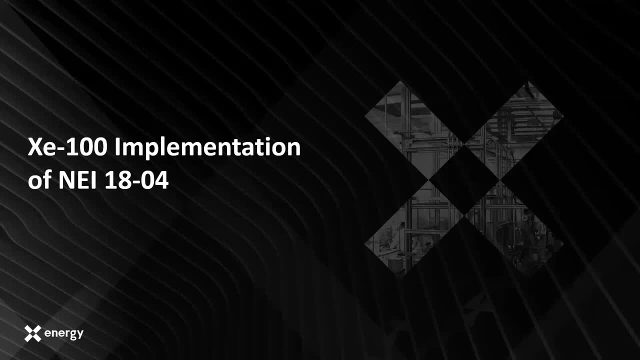 But I'll talk a little bit more, in more depth, about some of the things that we've learned, some of the processes we've put in place, et cetera. So we'll use that as the discussion point. All right, Great. 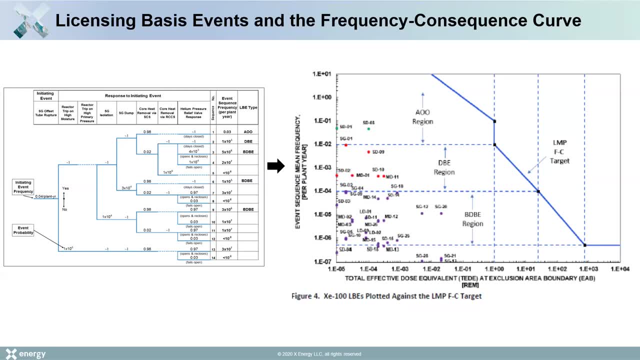 So, and the way that I'm going to structure this is walk through the three main elements of NEI 1804 and talk a little bit about you know how we've implemented it and what we've learned from it. So, again, the three major elements are the selection of licensing basis events, the classifications. 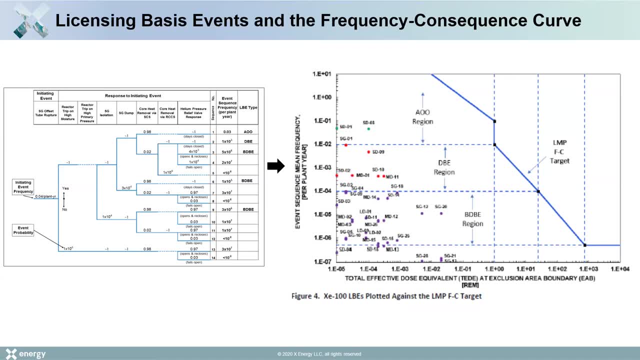 of structure, systems and components and the evaluation of defense in depth. So we'll start a little bit with licensing basis events. So the picture that you see here comes from what we know is our phase zero PRA. it was an initial PRA that was performed for the preconceptual XE100 design. 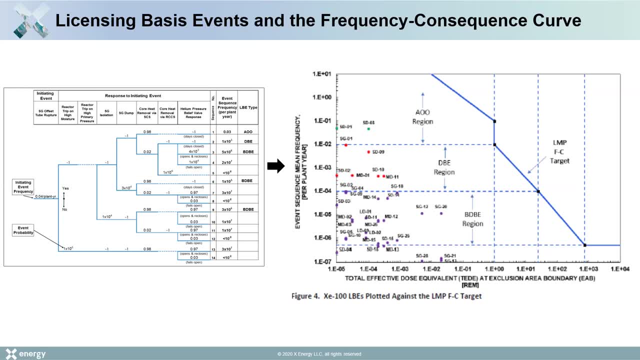 And on the right-hand side, here is the LMP frequency consequence target. It's the same thing that's in the NEI 1804 process. So for those who aren't familiar, you know this frequency consequence curve really serves as the target that you're seeking to stay less than. 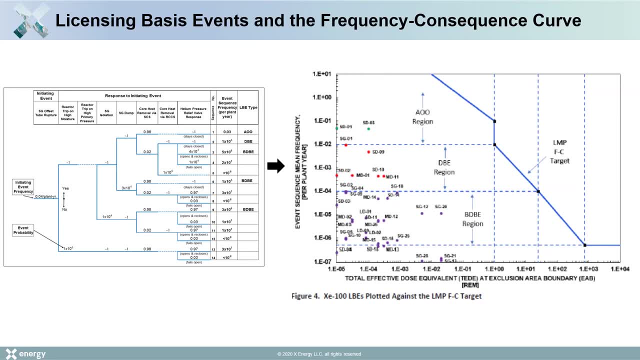 We're: on the Y axis is the event sequence frequency and on the X axis is the total effective dose equivalent at the exclusionary event. So again, you know these are the changes that you can do. But the next slide starts. you know this particular sequence frequency in your data. 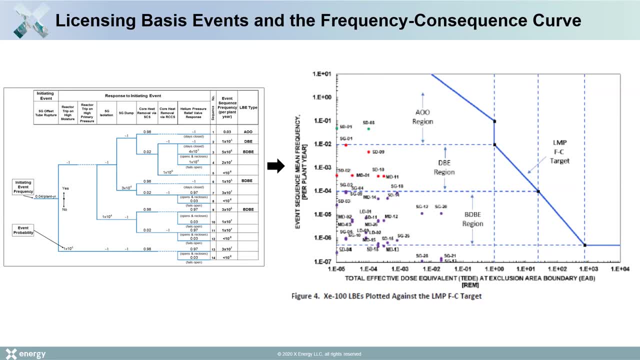 pumping data. So you take these two sequences And again you take the sequence frequency and you take the risk significance. You take the sequence frequency and then you take the risk significance. So we set Covalent to match the PRA and the FTC. And so you see that here the frequency on the PRA is higher than it is in the Hoxh wert. and then you take the frequency on the PRA, and the PRA is higher than it is in the Covalent. 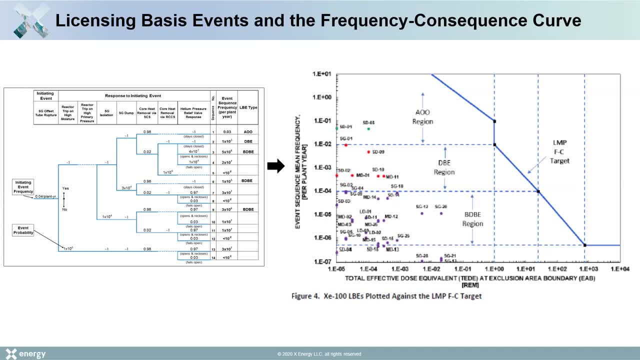 And that's the point of the sequence frequency. Now we're going to talk a little bit about a little bit more about sequence frequency and how we can hit those with the frequency of a PRA that's in our data processing database and just kind of auspices us out of the picture. 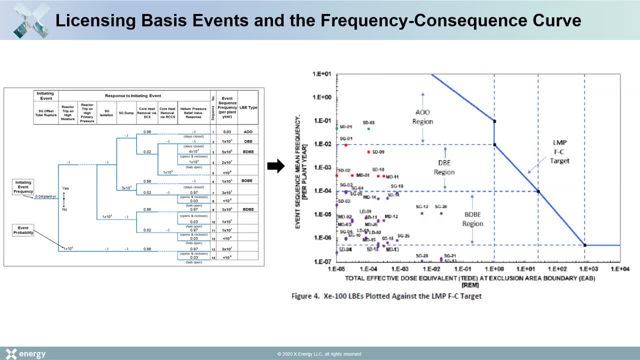 you know the safety case for the XC100 is very good. You know there's large margins to the target and even large margins to the to the frequency consequence, sorry to the risk significance line, which is again two orders of magnitude lower than this. You know with respect. 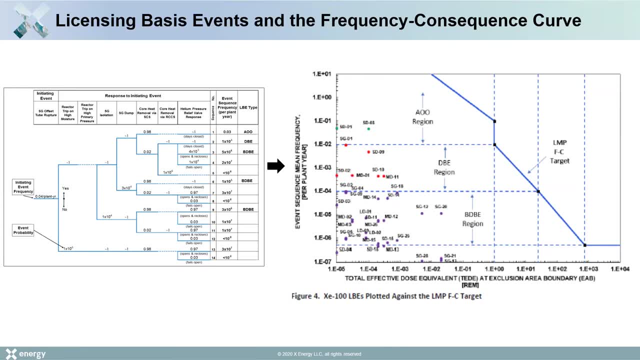 to going through the generation of licensing basis events. you know I would say it's you know nothing terribly controversial. I mean it's it's you know. you have the plant design. the plant design evolves. We're following the ASME non-lightwater reactor PRA standard. 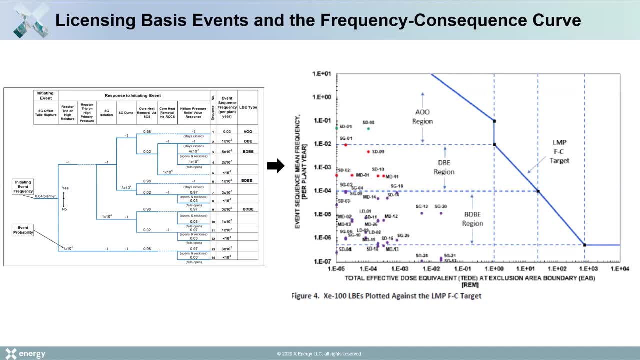 and you know, building the event sequences based on the information available to us. But even in this original state, I mean the original phase zero PRA that was developed was, you know, I would say it was based a lot on past HTVR designs with insights from the XC100.. 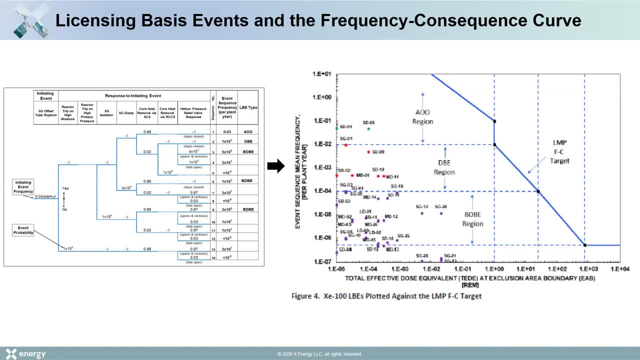 But even even with that, at that design stage and using that initial information, there were a lot of insights that could be gained from the PRA. As a matter of fact, that was one of the things that helped to select the use of two circulators. 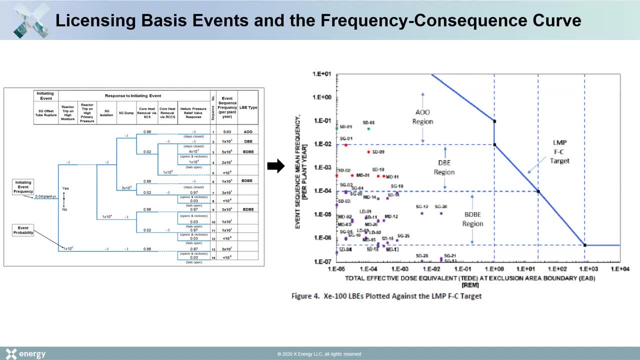 for the design And also inside the, the steam generator, the helical coil steam generator. there are two, two bundles, And part of the reasons for that were for trying to put sequences where you lost forced circulation out of the AOO region, And the AOO region is defined as the 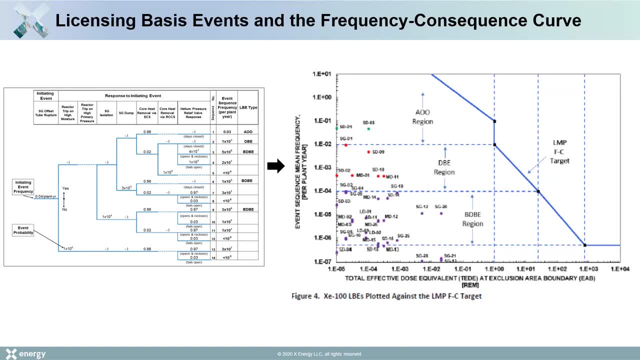 region frequency above 10 to the minus two per plant year, the DBE region between 10 to the minus two and 10 to the minus four. And the DBE region is defined as the region frequency above 10 to the minus four for plant year. And so there were even even with you know, say, you know taking 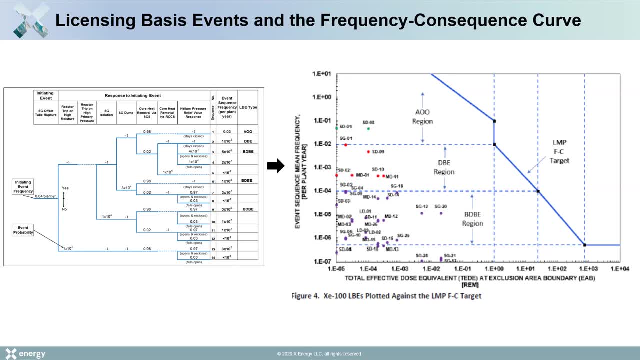 the compendium of knowledge from HTGRs and sort of making a more generic PRA. you know we were able to leverage that information to make some very important early on insights As the design and the PRA have continued to mature- and they've continued to mature substantially, I would say. 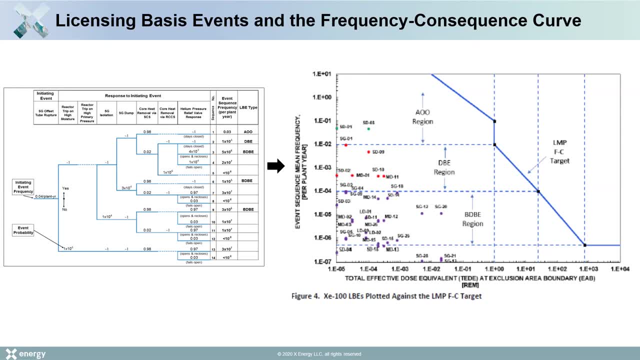 one of the major factors that we've been able to do is to make sure that the PRA is able to communicate with the design team, And I think we found, in implementing this process, it's a key challenge is, you know, making sure you stay in lockstep with the design. You know the design. 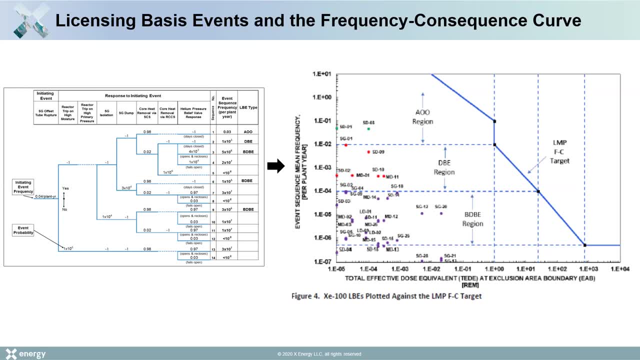 evolves very quickly in these stages, during the conceptual and preliminary design stage, And I would say, sort of at the beginning, it's really what we found is it's really important to set up clear communication between the, you know, the PRA and licensing teams and the design teams. 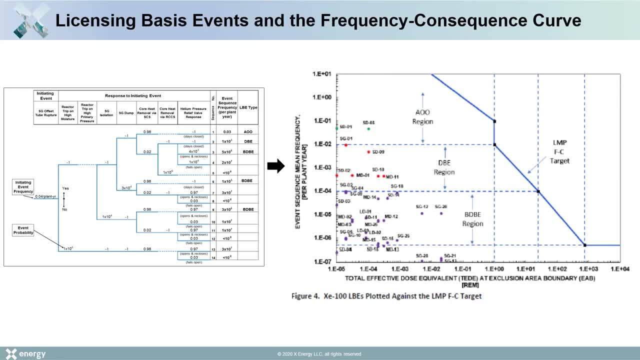 to make sure that PRA information is communicated, it's communicated in the right way and that information can then be taken and fed back into the design. But I would say that the design insights that have been coming out of the PRA have been very well received and very well. 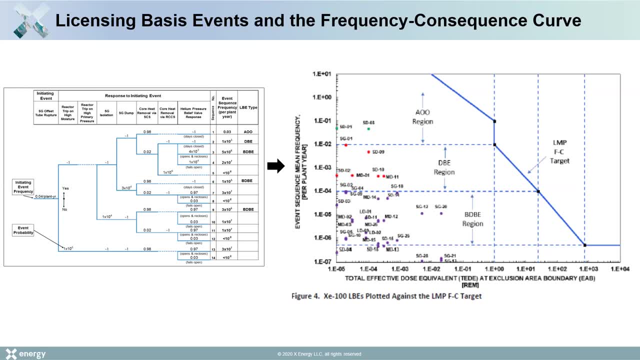 embraced by the design organization. I would say they're sometimes almost hungry for it. I think that you know people are really very interested to make sure they understand all the key considerations they have to make in their design. I think we find good exchange of information. 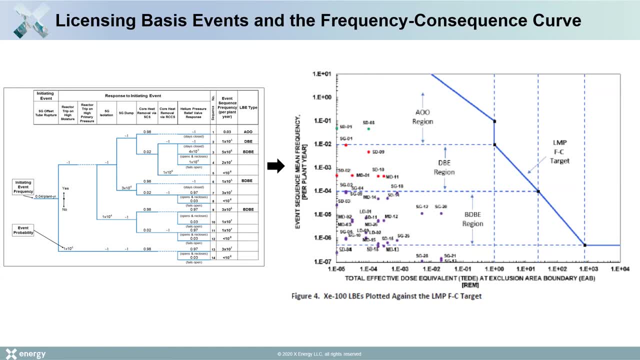 One of the things that we did very early on in the process to try to help educate people on the PRA, what you could learn from it, et cetera- because you know a lot of the people that are working in the design organization don't have a PRA background- is that you know we held sessions. 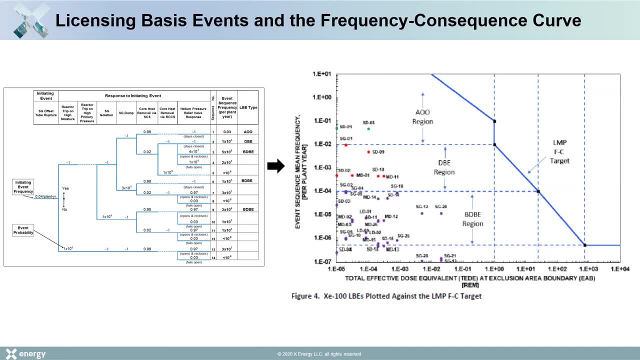 with the engineering team, reviewing with them this, at least at the beginning, this initial phase zero PRA, describing the major events, what their importance is, what their importances were, you know, getting feedback from them on differences in the design they were thinking. 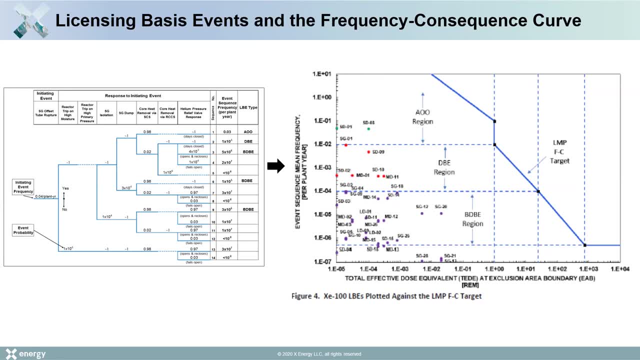 relative to what was assumed in the PRA and really served to have some really good integration and communication. So, you know, having those kinds of interactions we found to be, you know, really quite useful, And I would say almost, especially at the beginning of this. 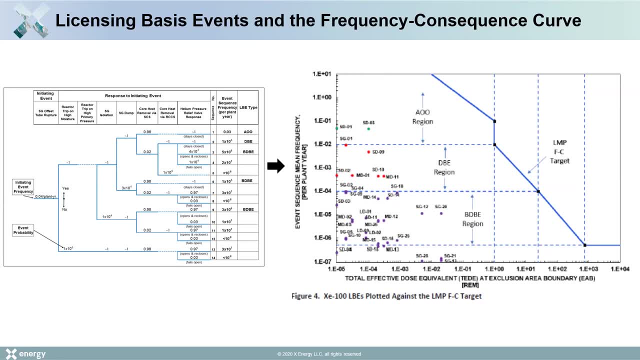 process. you know, one of the things that this does is it also just serves as a knowledge management tool, because if you think about the PRA, there's a lot of information heavily condensed and packed inside there Regarding the safety case of these kinds of plants, and it actually served. 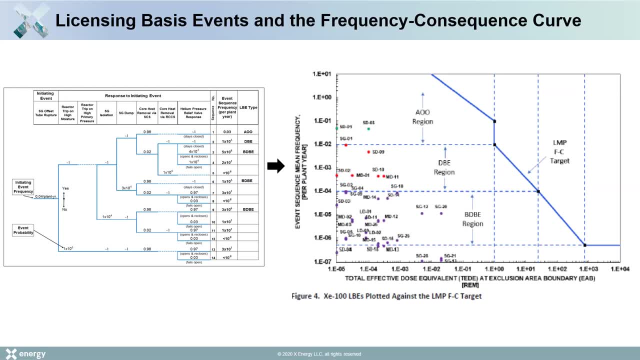 as a training tool to help people better understand the safety case of the reactor and what's important. So, again, this initial PRA that you know again wasn't, I would say, very heavily informed by a very specific XC100 design, but you know the designs upon which. 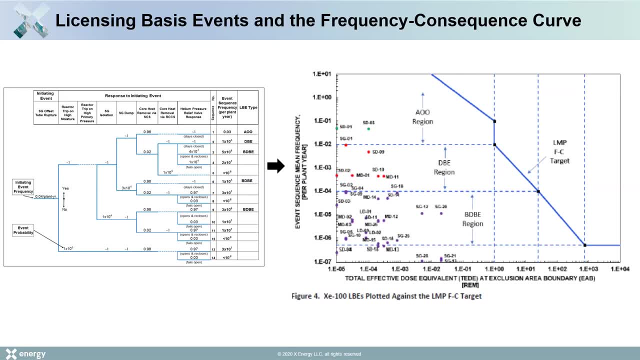 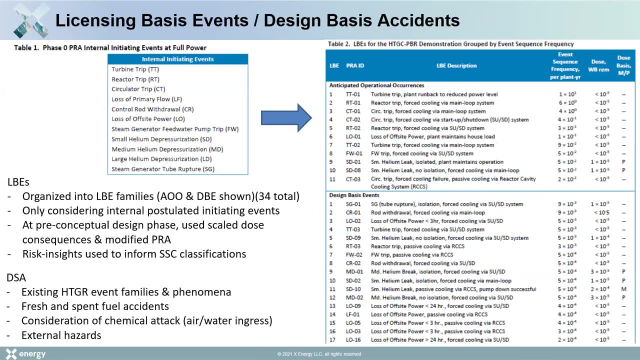 it's based, you know, served a very valuable purpose in informing the design as well as helping to as a conversation starter with the design organization. So you know, so again, the PRA that was developed and then it has again. 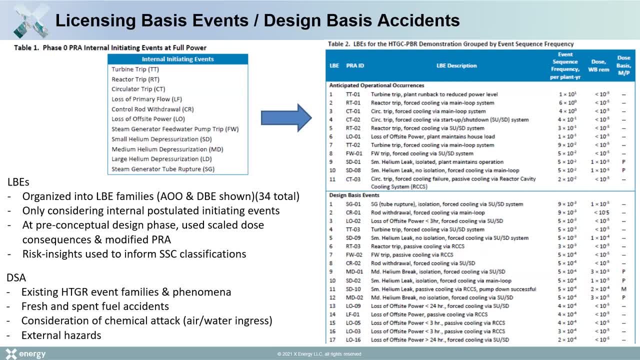 has continued to be furthered And at the time when the initial phase zero PRA was developed, there were 62 licensing basis events that were identified, so 62 scenarios on the event tree, and we used several different initiating events that were evaluated that I would say are: 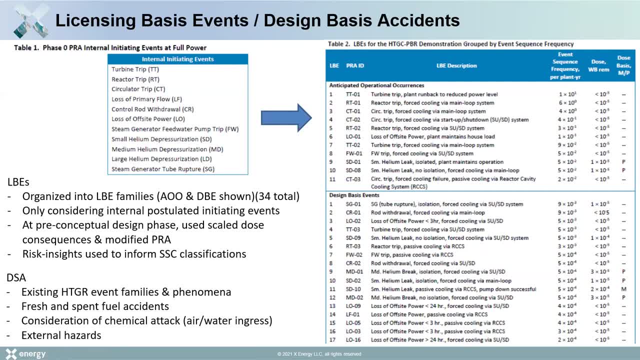 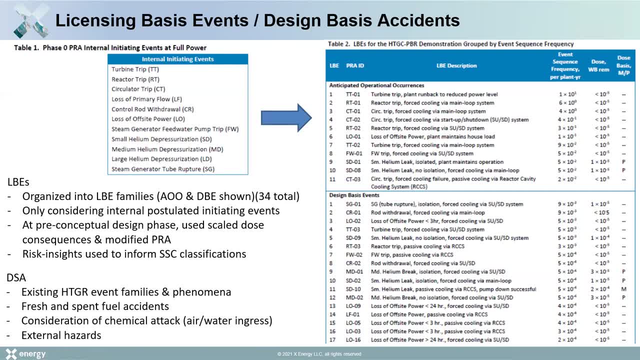 circulator trip, loss of flows, control rod withdrawal, accidents, loss of offsite power, loss of feed water, depressurization events of various sizes and steam generator tube rupture. As the, as the design has evolved and the PRA has evolved. 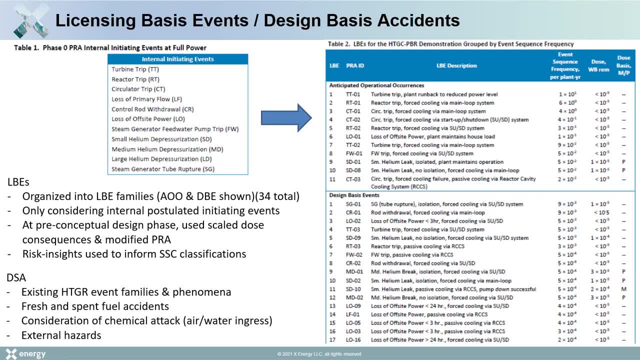 you know, one of the things that we're starting to factor in more, things like support systems, you know. so these, these events, I would say, are really very, you know, primary system and secondary system focused, But obviously there's a lot of support systems which feed these And I think 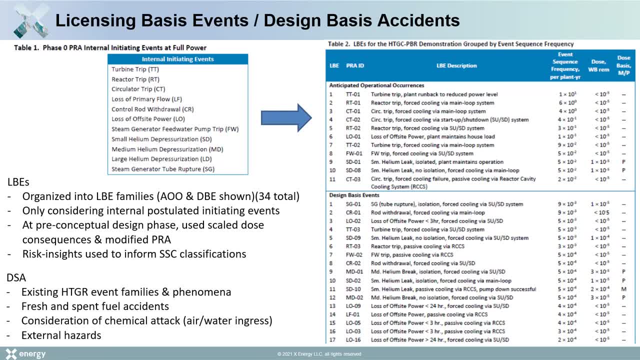 we're seeing some insights. that's very similar to the kinds of insights that light water reactors saw when they looked at initial PRAs and, and you know, saw the importance of things like component cooling water and service water right. So those you know understanding the relative importance. 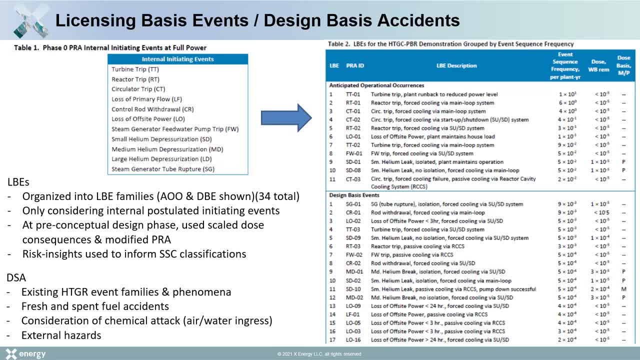 the risk of those, of those support systems is starting to become an important factor to us. Now, again, I say importance. you know importance to risk and when the overall risk is very low. so I'm speaking in a relative basis, but we're starting to get a better idea of how those 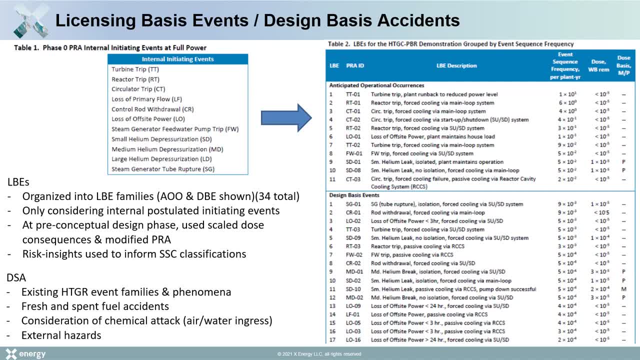 systems you know are important to safety, as we get deeper into the PRA and start building out a PRA that's more XE 100 specific and goes deeper down into the systems And some initial insights also that came out of the PRA, is you know? 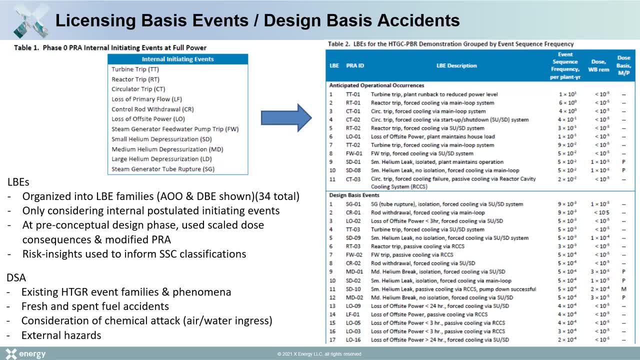 I mentioned that there were some design decisions that were made at the beginning to try to limit the number of sequences where you were relying on passive cooling. you know, try to to maintain active cooling in the AOO region as more of a defense in depth philosophy. 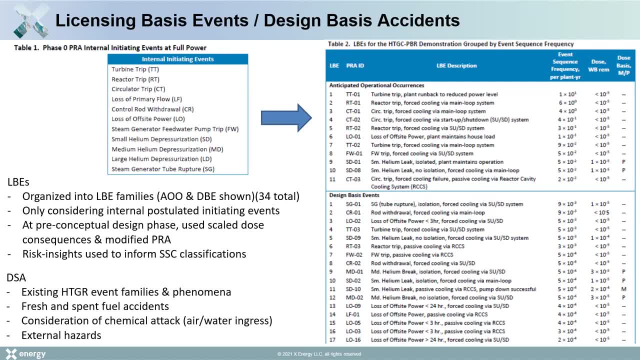 And I would say, when this initial PRA was developed and even some more recent work, you know we identified some scenarios where, you know, that was not happening to the degree we wanted it to. Now the plant can, you know, obviously rely only on passive cool down. We don't need the active systems. We just don't want to be relying on it all the time. right, You don't want to be relying on passive cool down. Your temperatures, you know, get much higher. You'd rather not be cycling the plant that much. 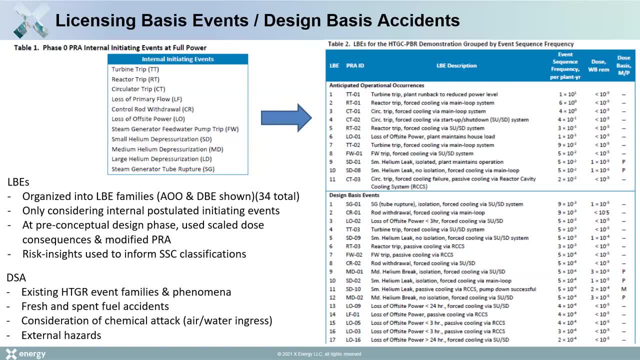 It's a lot harder to get the plant restarted if you need to. So it's just a lot of benefits for staying on active cooling And the PRA was helped to identify that And it's also helped to communicate with the design team. you know what design requirements. 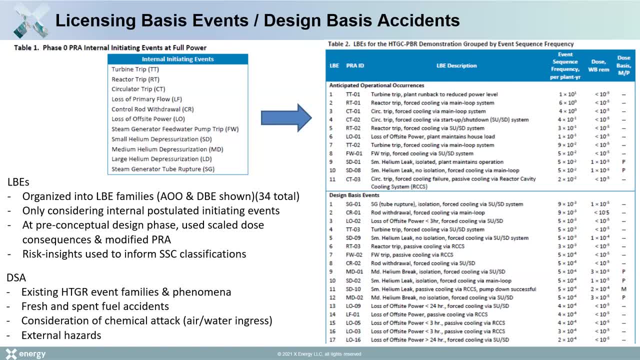 are going to be necessary for various systems in order to be able to, you know, meet the targets that we want, We were trying to achieve. So, you know, we found, you know, I would say that we've utilized PRA. I think very. 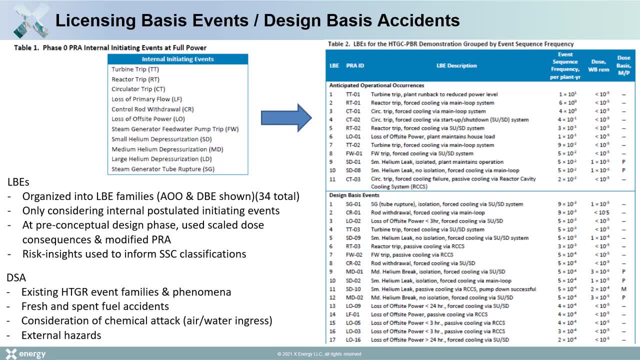 heavily during the design process to provide feedback into the design And you know the system engineering team is reaching out to us quite a bit to understand. you know what's the PRA saying and what are the insights that they're telling us. 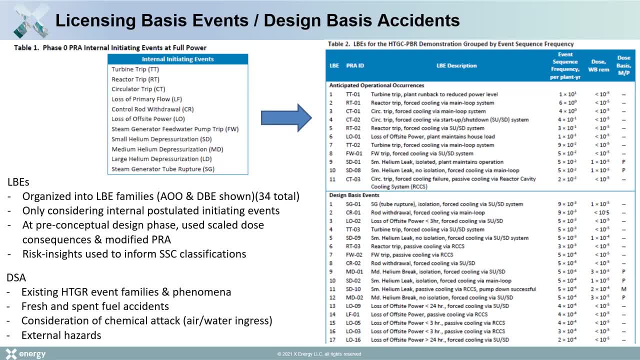 So I think over time we've gotten a lot of really good integration, developed a culture of people, People who understand that this process can really give them the insights that they need. You know, and from the licensing basis events, you know. so you know there are sort of 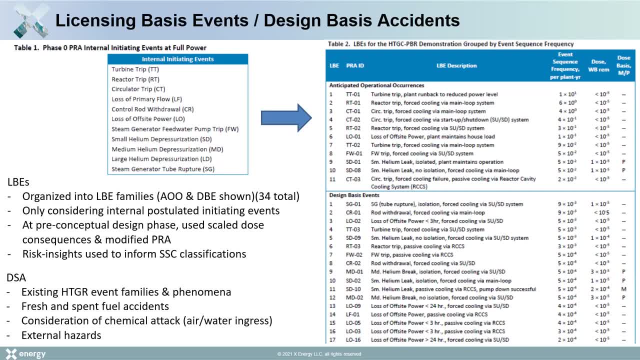 two pieces to the overall process. right, The LBEs you know, tell you sort of the PRA story and you know how you compare on the frequency consequence curve. But you know there's a deterministic side of this and that's the development of design. 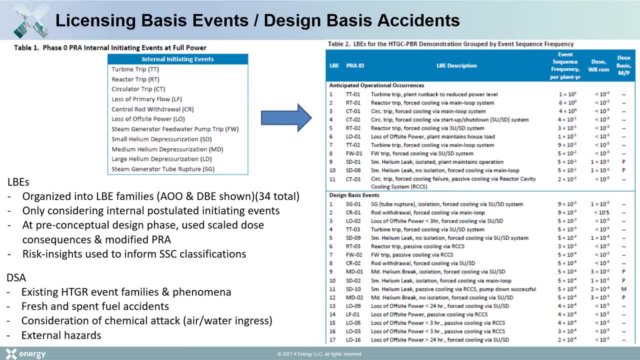 basis accidents And for those who aren't aware, you know so, design basis accidents are something that you derive from event sequences in the design basis event region. So if you look at, you know the sequences here. this is the DBE region, between 10 to. 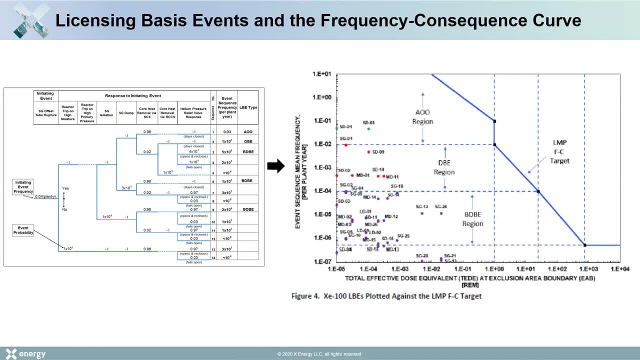 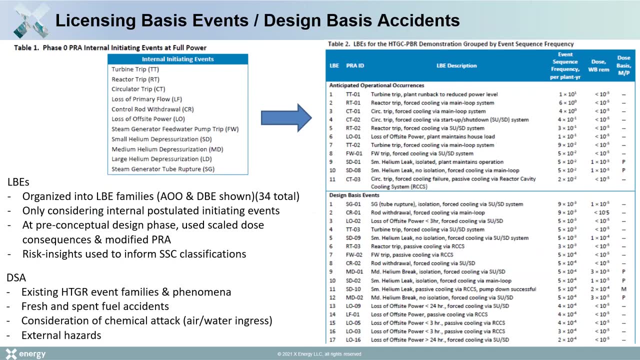 the minus 2 and 10 to the minus 4 per plant year. You know, you take those sequences and you develop design basis accidents by crediting only safety-related SSCs, right? So you and I'll talk a little bit about, you know, our initial assumptions on what. 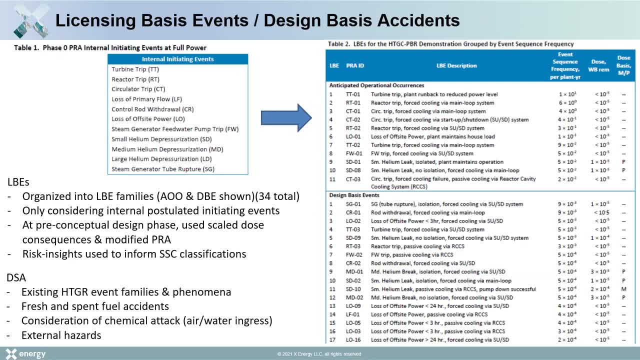 those systems are in just a moment. But you know, you understand that You only credit safety-related SSCs and then you run accident cases that are include the typical deterministic penalties, you know treatment of uncertainties, et cetera. 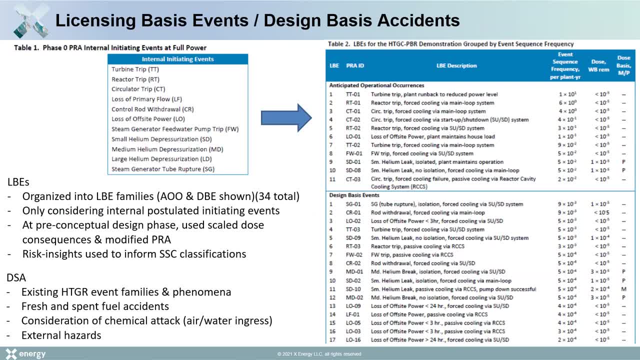 They go in with that. And I would say one thing that's been interesting is that concept confuses a lot of people When you talk about LBEs and DBAs, and especially when you start saying DBEs and DBAs and the 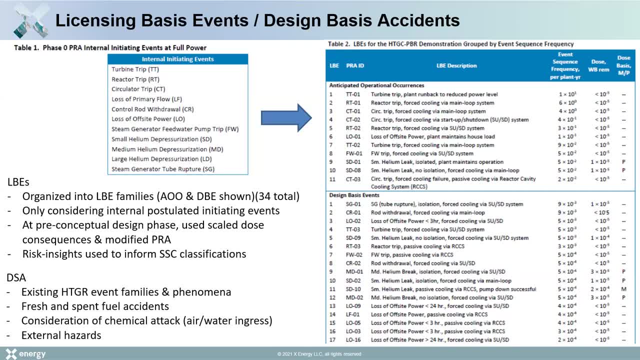 different assumptions that go into them of what they mean. right, because the DBAs are meant to be compared against regulatory dose limits, whereas the LBEs really help to inform you on your classifications. people really struggle with that And I think you know. I've had to explain that you know numerous times. you know. 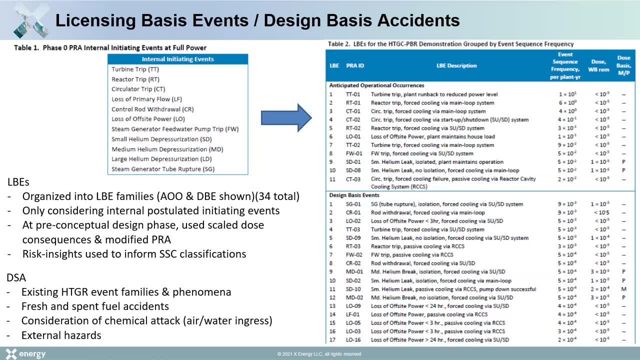 and I very possibly could be explaining it badly, but you know, trying to make people, help people understand the distinction there and why one or the other is important, I think has been an important lesson for me in you know how to communicate this to those who. 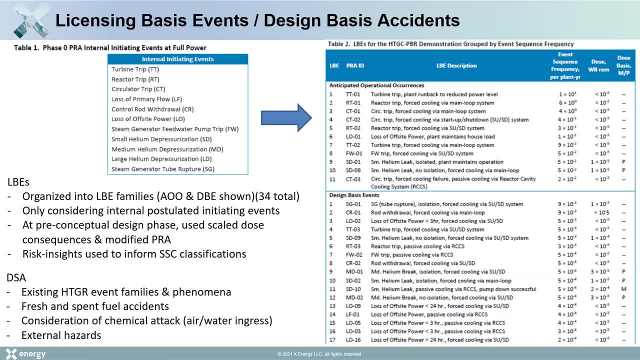 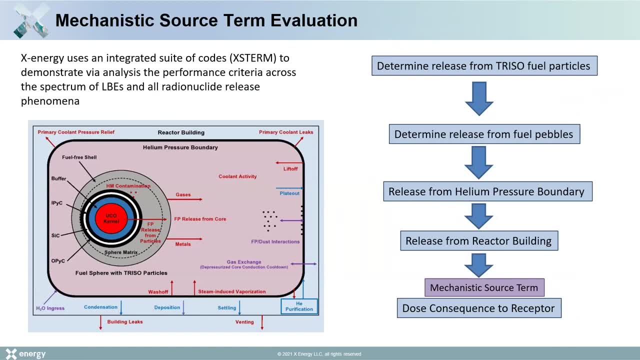 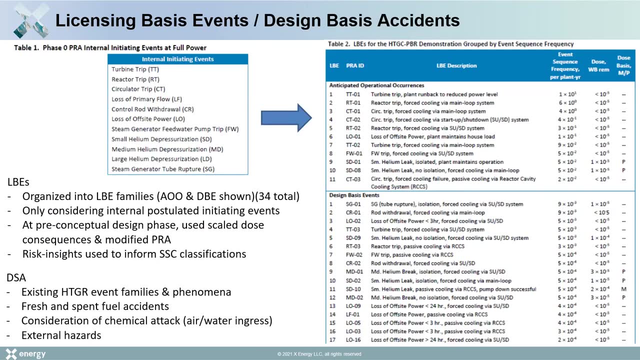 aren't necessarily practitioners in this, So you know. so what I've sort of said so far is really related, I would say, to the PRA side of things. So the development of the event sequences and the initiating events, you know. but there's 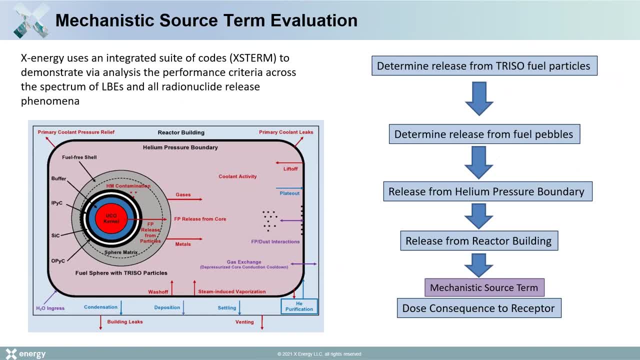 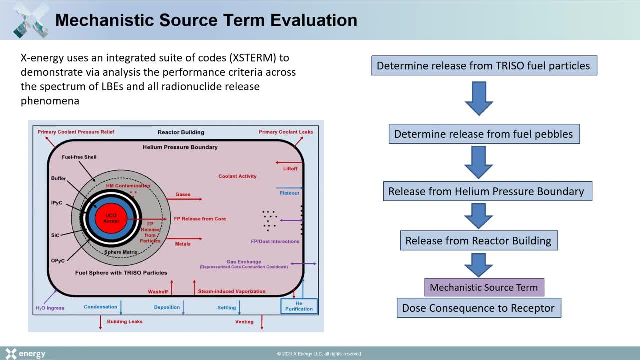 LBEs and the LBEs and the LBEs, to be able to make estimates on the consequences For. but more recently we've been developing more detailed mechanistic source term evaluations that are XE100 specific, And XEnergy has developed an integrated suite of codes known as XS term to model all of. 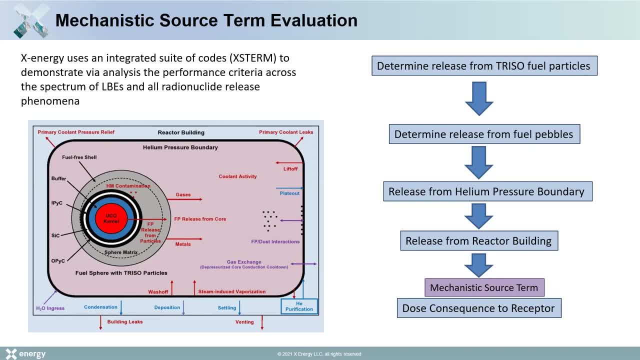 the various phenomena that are important in an HTGR design and to be able to capture those in the LBE evaluations, Because in the LBEs we want to try to treat the LBEs as a set of values that are important. So we've started to develop a set of values that are specific to the LBEs and the LBEs. 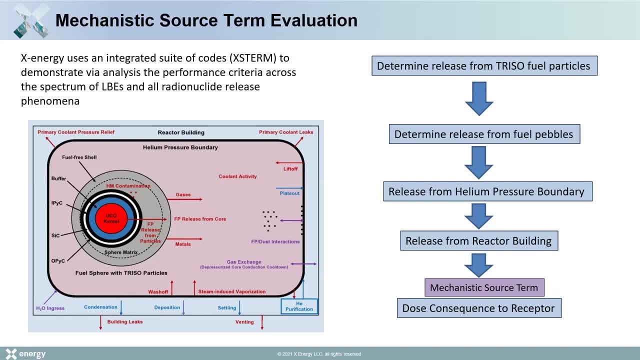 and the LBEs as a set of values that are specific to the LBEs. The physics is as best as we possibly can without dealing with conservatisms, And we really need a good mechanistic source term evaluation tool in order to be able to. 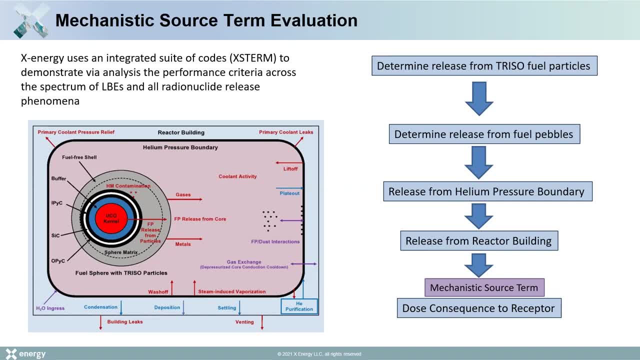 do that. So to give you an idea of the various physics that the tool is handling- and again, I don't know everyone's background, so I'll briefly just kind of go over the key aspects of the HTGR mechanistic source term case. 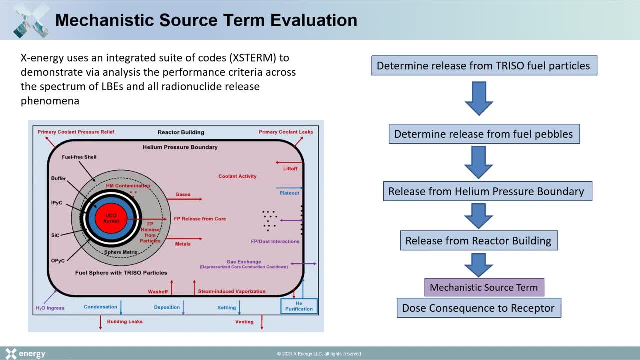 So the major safety case in the HTGRs is the triso fuel, Where most of the fission products are retained inside the kernel and within the silicon carbide layer that acts as the pressure vessel And as part of the XC100 design. even for our worst accidents, we don't expect any significant. 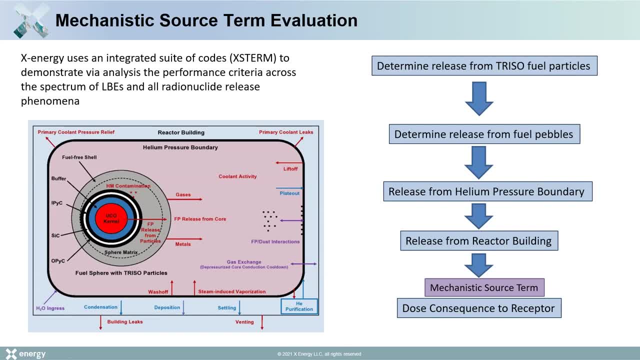 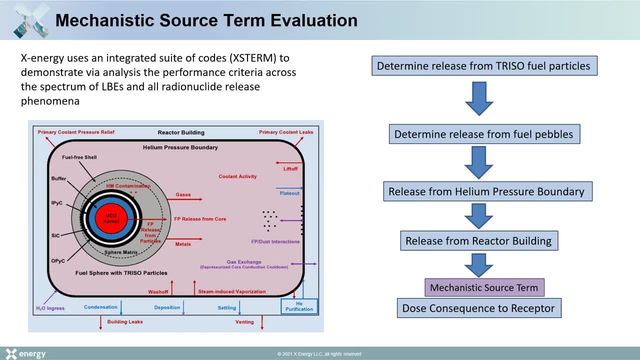 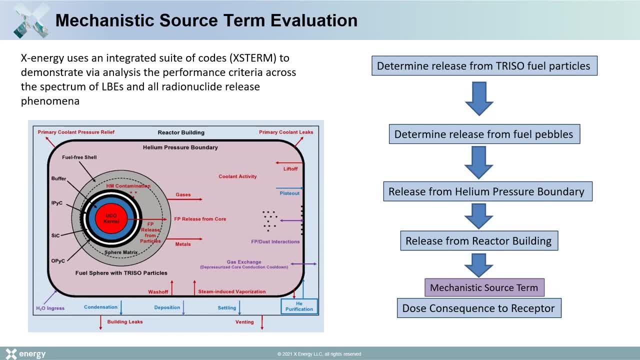 And so we have the XS term code can model the diffusion of fission products out of the kernels for those failed particles, the diffusion of heavy metal contamination, the diffusion from the graphite pebbles and release into the helium pressure bound Okay. 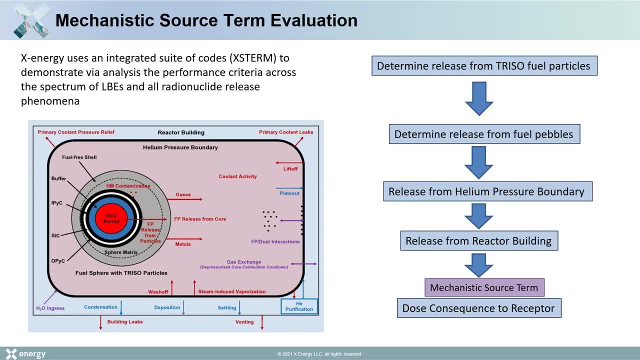 So that's the first step, The subsequent circulating and deposition and liftoff inside the pressure boundary And then, in the event of a depressurization, you know, the ability to track the radionuclides as they go out into the reactor building and then out into the environment. 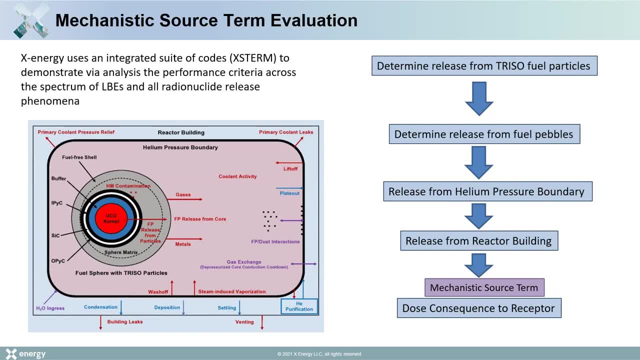 And there are also mechanisms inside the tool set to be able to handle moisture ingress and air ingress effects as well, such as wash off, steam off and other oxidation effects that can occur. So you know, as part of the excess term evaluation, you know we can evaluate the triso fuel release, we can evaluate the fuel pebble release release from the pressure boundary in the building in order to evaluate those consequences. 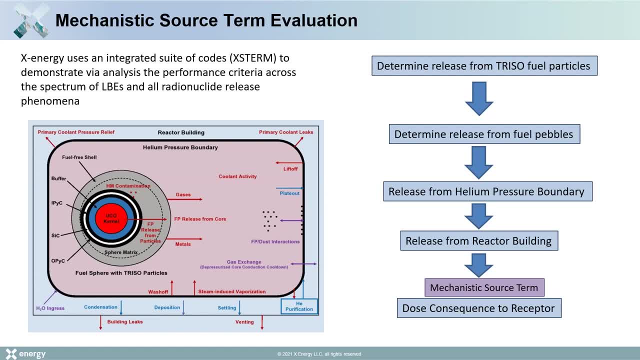 And so we don't necessarily do this for every event sequence. It's a lot of physics to be calculating And so we run it for a family. you know we run some cases on a family of event sequences But we can go evaluate the specific mechanistic source term for each scenario. 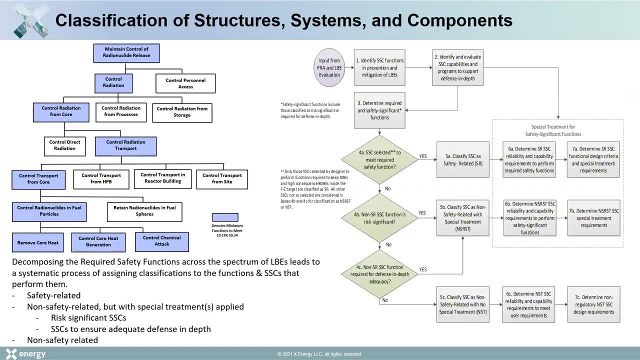 So that's one of the things that we need to cover. Sorry, is there a question? Somebody just off mute. I'll keep going. I think we are hoping that people who have questions will use the chat function while you're speaking, Okay? 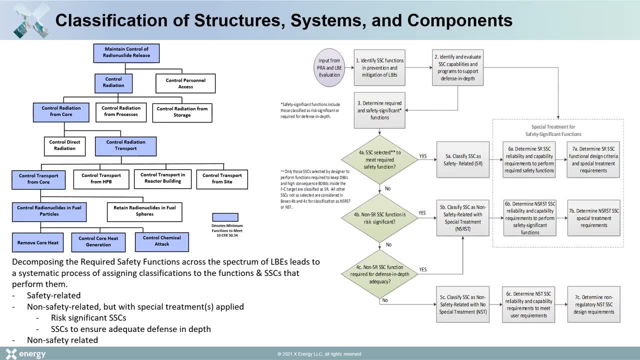 Okay, so I'll move on. next to the presentation, The next piece of the process and that's the classification of SSCs. You know so at a high level. you know NEI 1804 has three different classifications in it. That's classifying as safety related, as non-safety related, with special treatment applied, and then you know non-safety related but with no special treatment. 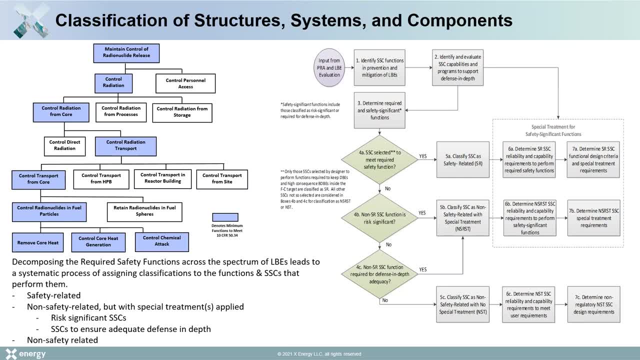 And there's a process inside NEI 1804 for you know what leads you to those various classifications, You know, and for the safety related piece, it's really about those SSCs That are needed in order to meet your required safety functions, and that's. I'll describe that in a moment. That's described by this tree over here. You know what are the minimal functions that you need in order to ensure that you meet your offsite dose limits. 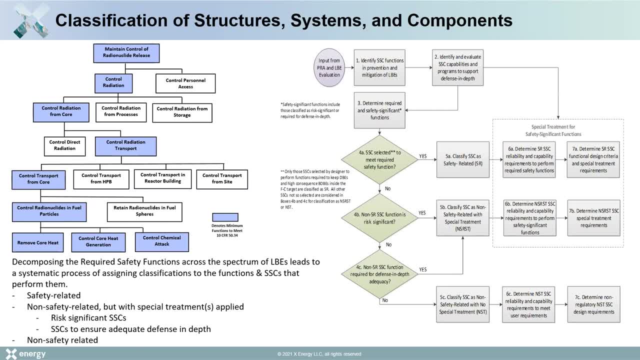 For non-safety related with special treatment, which I'll refer to as NSRST. there are really two ways that you get there. One is by the SSCs being risk significant, So contributing overall to one of the quantitative risks, And then the other is through SSCs that are necessary to ensure adequate defense and depth. 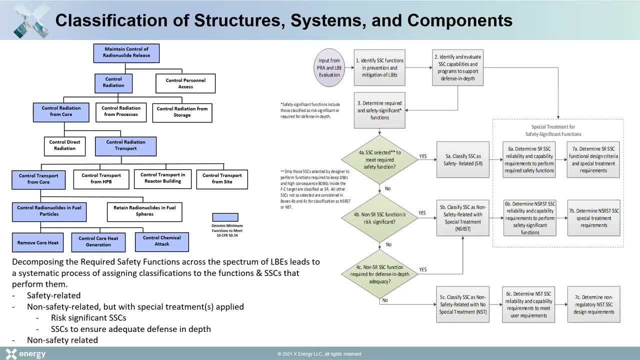 So I'll talk a little bit about the. you know the safety related systems first and then I'll talk about the. you know the process for selecting NSRST. So, as part of again, what I'm showing here on the left hand side is coming from the comes from the LNP pilot that that we're using. 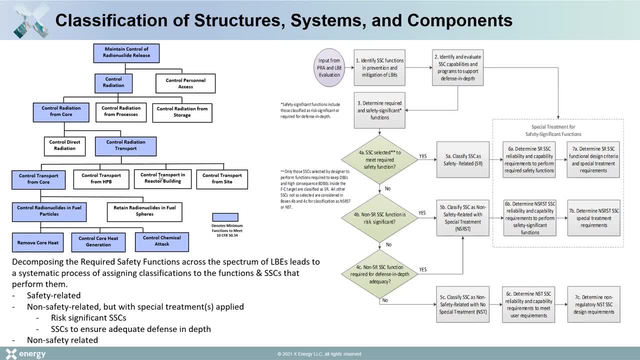 That X Energy took part in and this has evolved some, as we've as our knowledge of this, our particular design has, it's also evolved. But basically, you know you start at the top level, you know trying to. you know our ultimate goal is to control radionuclide release. 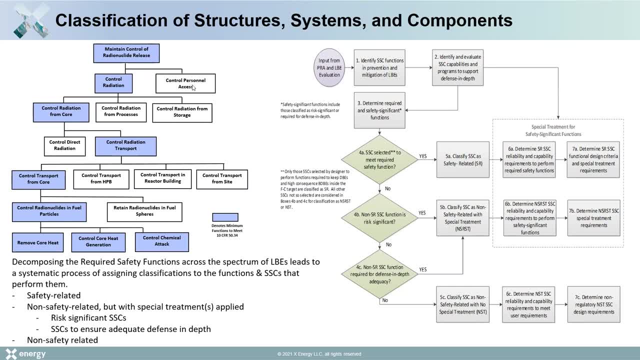 You know there are various methods that you do that for various sources of radionuclides. You know you have to control radiation. You control the radiation itself, You control access to the radiation. Controlling radiation from the core is compared to processes and storage. 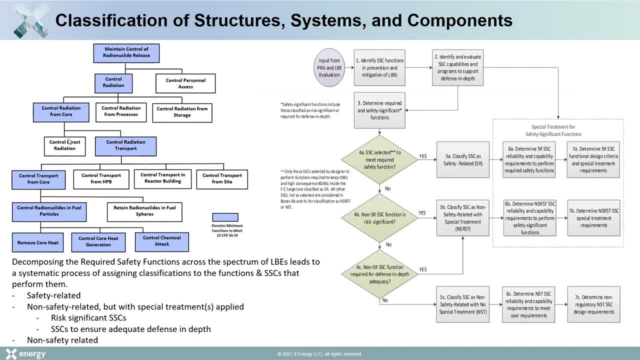 Controlling radiation: Radiation and trans radiation transport versus direct radiation. So this is something that will be handled with something more like shielding versus radiation transport from the core, And then you get into the various mechanisms for how you control transport. And these, these blue boxes here are ones we've denoted as sort of the minimum necessary in order to meet the the offsite dose limits. 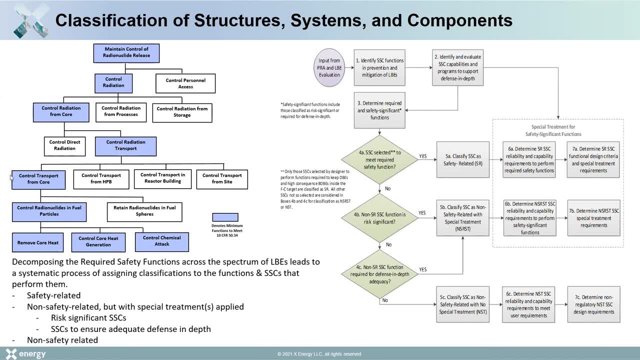 And so what? and when you get down to the bottom here, right, so we're focusing on controlling transport from the core, controlling radionuclide And the fuel particles, and really that's about maintaining particle integrity that's governed by temperature, which is a balance between removing heat and generating it, and then also controlling chemical attack and that really comes from the steam generator to rupture accidents that can occur and moisture ingress events. 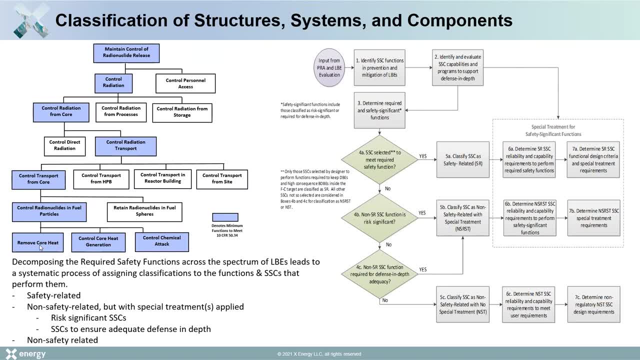 So this is sort of the the minimum set of functions that we have to meet in order to be able to guarantee that we can satisfy offsite dose limits. and then you use this in order to be able to select leaders. So you can see, here we have the potential for the SCC, as you know. so for the XC 100, you know, clearly, controlling radio nucleides and fuel particles- well, that's going to be the fuel particles for removing core heat and controlling heat generation. on the control heat generation side, you know our work. we're currently looking at relying on the inherent reactivity only, right. so clearly, we have control rods for the core, but our current claim is that we don't need to rely on them in order to be able to shut down the reactor safely. 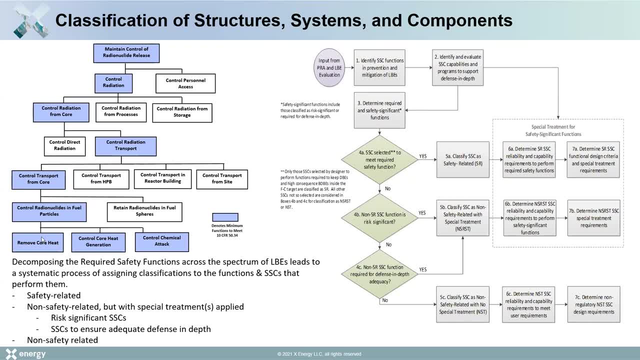 And then for removing core heat. you know we can remove it passively by conducting and radiating out of the vessel. And then for control, chemical attack. it's really about minimizing the amount of water ingress that can occur in a tube rupture event. So there are various mechanisms to do that. So you know. 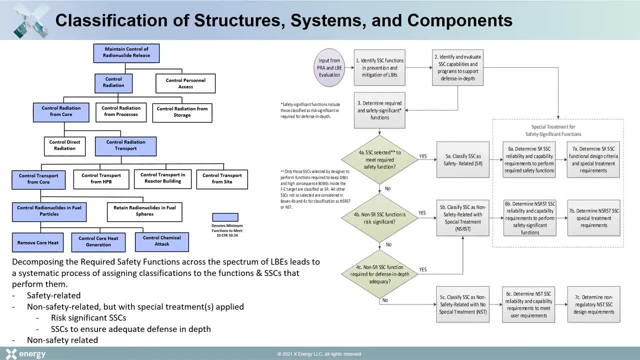 that really comprises the totality of the safety related systems, right, So it's a very minimal set at the whole point. you know there are four or five different, you know, safety related SSCs that we consider And really that's kind of not the controversial piece of it, you know, I would say 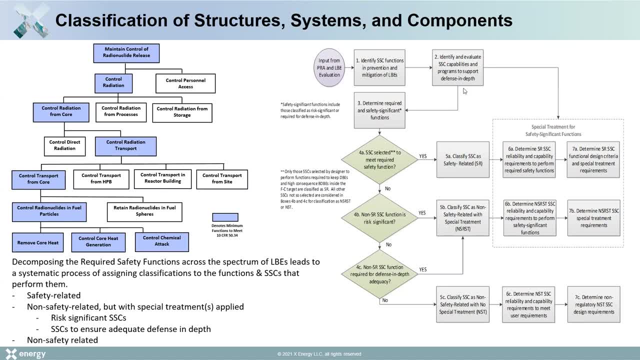 it gets more complicated when we get to the NSRST part. The one thing I will note is that, you know, while this is the minimum set of functions needed, that doesn't necessarily mean we're going to decide that that's all we're going to credit in the safety analysis. And I say that because you 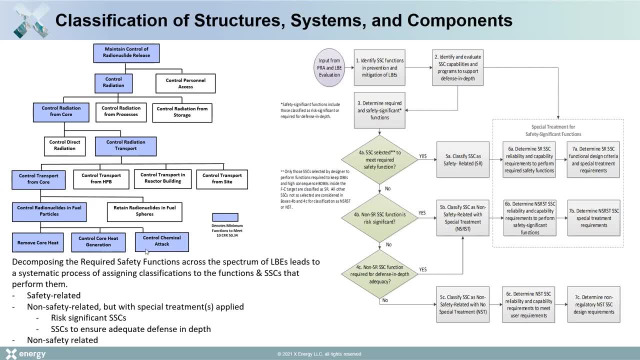 know I can, we can meet the dose limits by following this. But you know there's a balance between the two, And so you know there's a balance between the two, And so you know there's a balance between, you know, having margin during operation. it's really a margin. 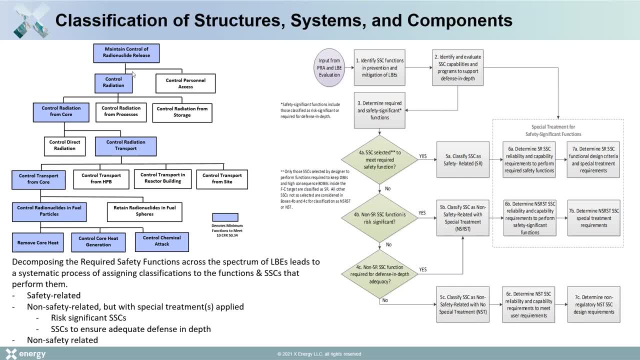 management issue right, As you credit fewer and fewer things. you know our doses. we can still meet the limits, but they're going to be higher than if you could credit certain things. But we may. you know it's possible to make a choice to say, well, I'm going to V&V my tools to model. 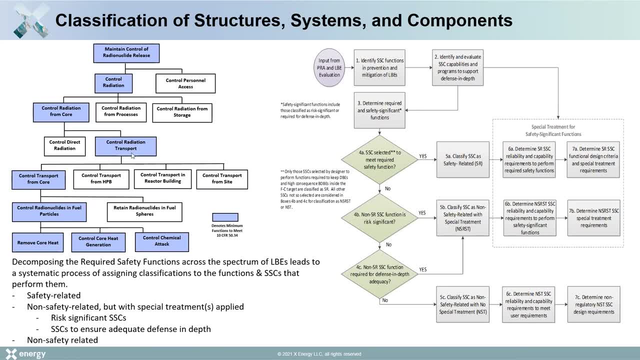 these phenomena a little more explicitly And I can take credit for them. that's going to reduce my doses, that's going to give me more margin and operations. it's going to cost me more upfront to do the V&V But you know I'll gain more margin operationally. So you know this is minimally what. 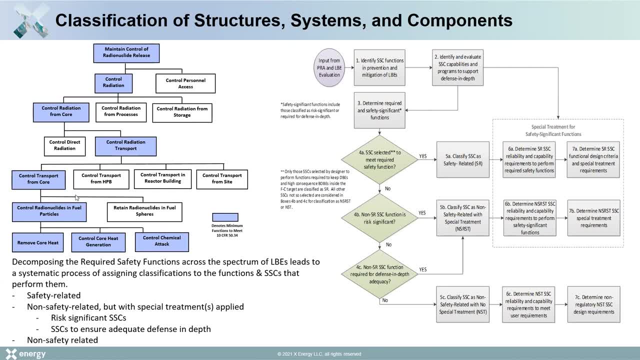 you have to accomplish. But I would say that you know we've had a lot of discussions about you know where do we want to use the margin we have? And I would say that's an ongoing conversation. I would say where it gets more complicated is in NSRST. That's really you know. if I have to say 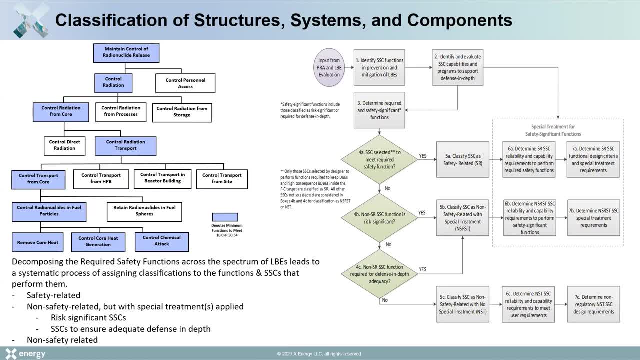 where our day to day conversations, where we spend them. it's always talking about NSRST, Because you know one. we have a very small set of safety related components And then, within the two ways to get to NSRST, either by being risk significant or having you know SSCs that 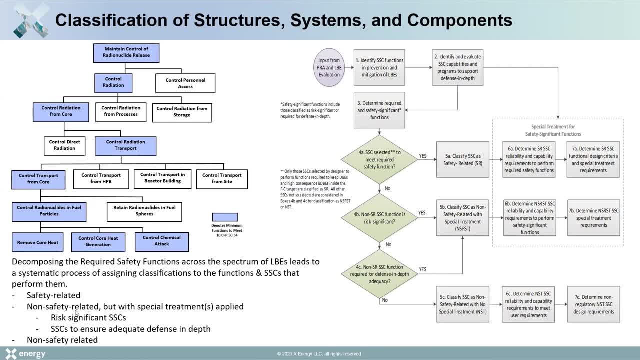 are necessary to ensure adequate defense in depth. we're not currently predicting we're going to have any SSCs that are defined as risk significant. Everything is really going to be driven by ensuring adequate defense in depth, So that's really what drives most of the work that we're. 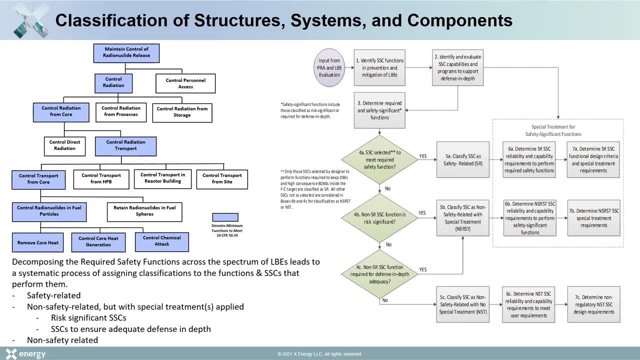 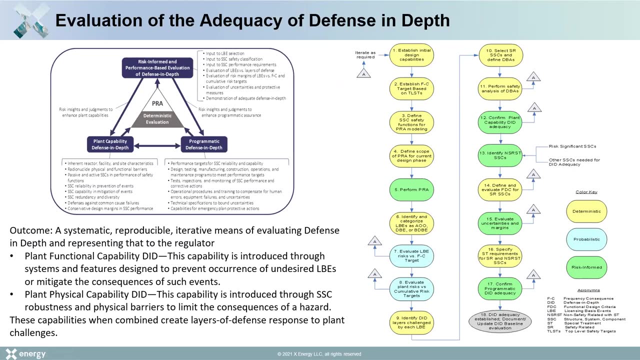 doing in terms of our NSRST classifications- See checking my notes. And yeah, I think I'll think that's good for that. And so, with respect to the final piece of it defense in depth, you know this, if you look at NEI 1804, you know it- it kind of breaks these three major pieces that I 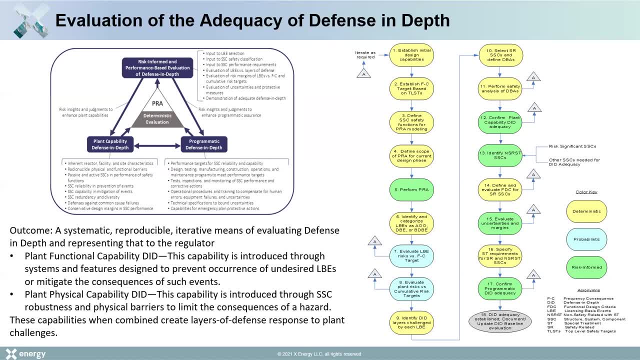 mentioned: selection of licensing, basis events, SSC classification, evaluation of defense in depth adequacy. you know it looks like three processes. it's not three separate processes, they're clearly intertwined. But I think one of the things that we've learned going through this is that you know, as an organization, you have to build a. 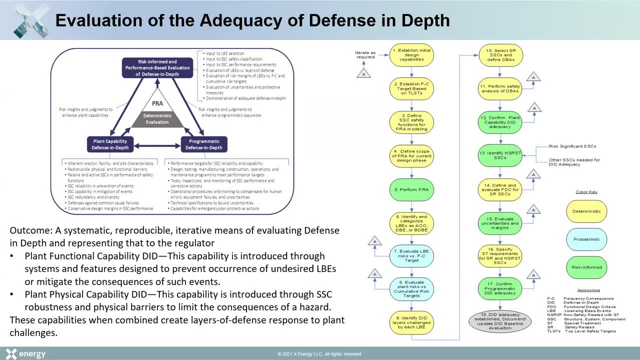 process right, And I think what I see these various pieces are is tools that you have to put together in the right way in order to work for your design. And so you know, we spend a lot of our time talking about defense in depth because, again, I think the safety related piece is fairly. 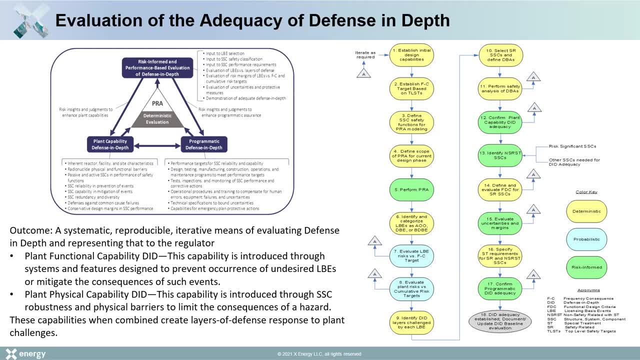 clear Like: you know we're talking about. you know we're talking about, you know we're talking. I think we have a good case for that In NSRST. we don't have. we're not identifying risk. 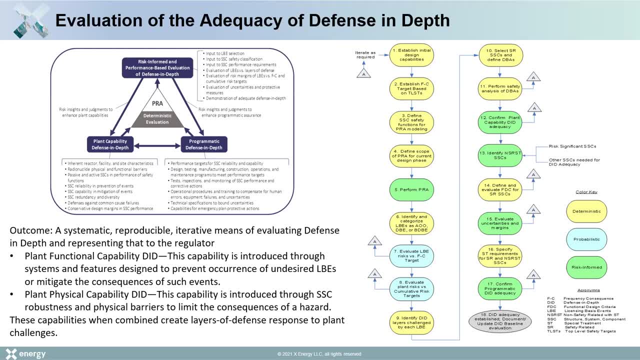 significant SSCs, And so really all the conversation is about defense in depth, And so you know, I would say, our defense in depth, adequacy and evaluation, it's really quite baked in with our SSC classification process, Because those are the major questions that we're. 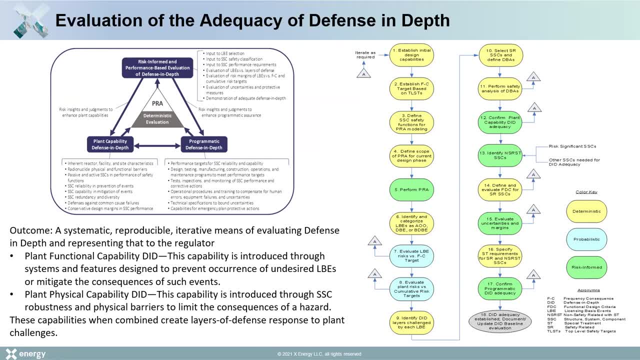 asking all the time. So you know we are looking at defense in depth on a regular basis, you know, making sure that, as we're making various classifications, that our overall defense in depth posture makes sense, And so in the end, you know, we'll probably run through the whole. 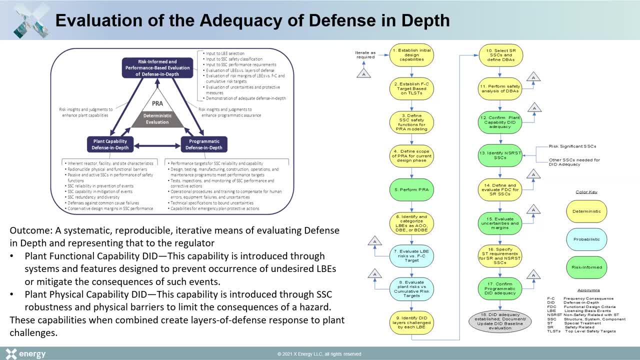 process to make sure you know at the end that the posture is what we want it to be. But I would say it's something that we found we're heavily integrating as part of the defense in the SSC classification process along the way And the way we tie all this together right. so the 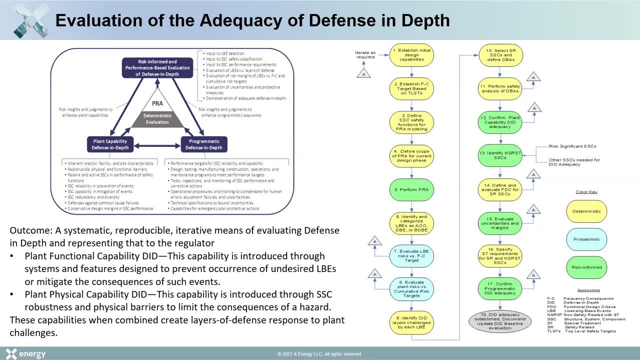 organizational way in which we go through the process. we're going to be looking at the implementation team, which is the team that I coordinate, And then we also have what's known as an integrated decision-making process panel, an IDPP, And so the implementation team is the one. 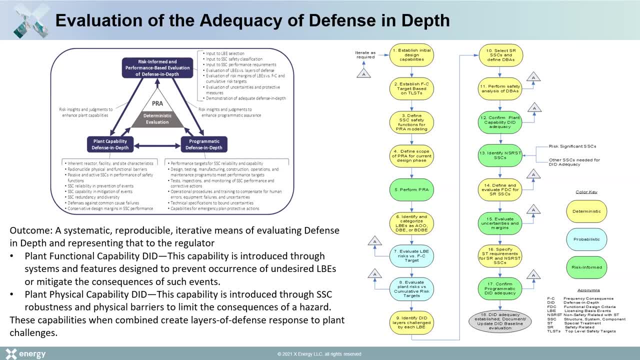 that's, you know, working with the PRA team. The implementation team consists largely of folks on our licensing team and some folks on our PRA team, And so they're working to work with the rest of the PRA team. safety analysis team pull together the information. I would say. 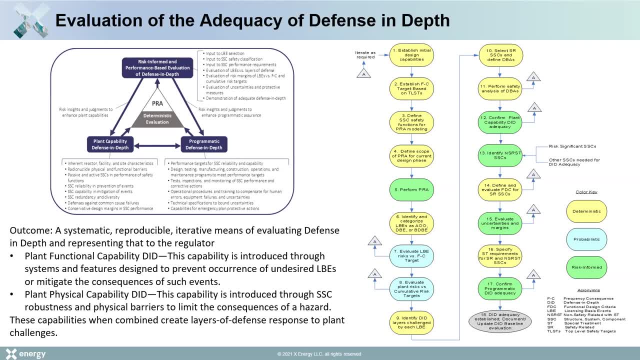 facilitate the conversation with the design team, because we try to really get our design teams heavily engaged in the process so that they buy into, you know, some of the recommendations we're making on classifications and special treatments, And then that is put together in a package and 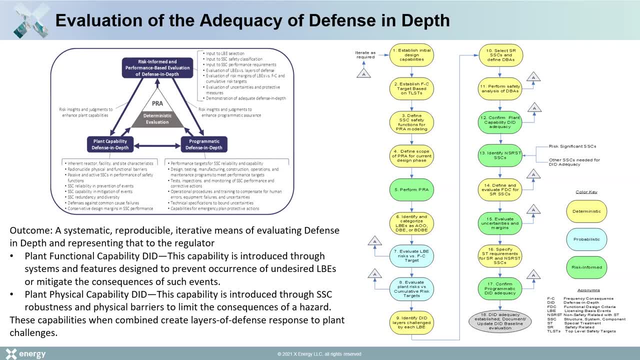 reviewed by an independent panel, which is the IDPP right. So they review it, They represent, you know, operations safety analysis, also represent PRA system design etc. And then they review and comment And approve the classifications and the special treatments that are recommended. 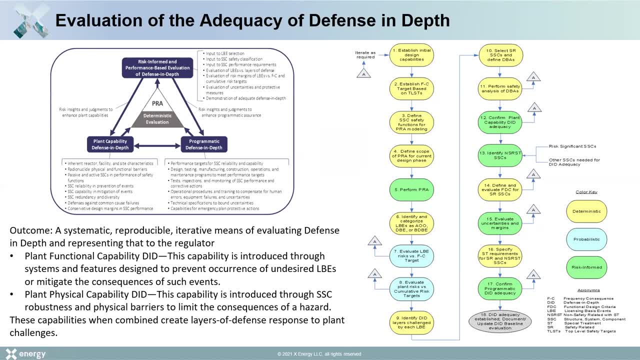 And the way that we have sort of proceduralized it, or we haven't exactly proceduralized it because we produce guidance. But you know, the IDPP was a charter established that identifies what the basic process is that X Energy is following to implement NEI 1804.. And then various guidelines. 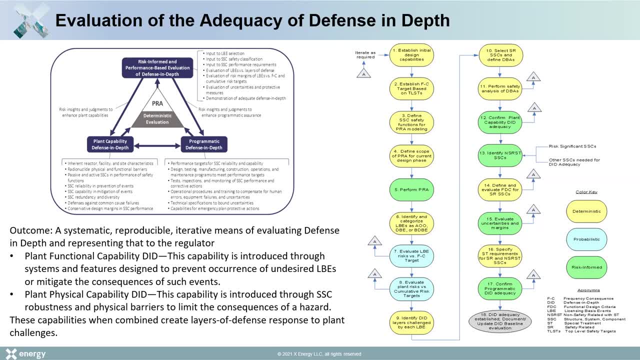 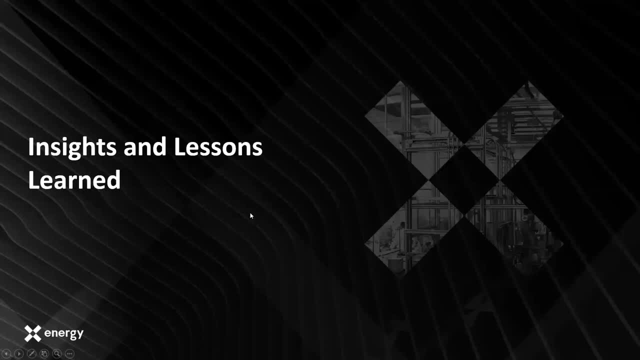 that give you know, to make sure that you know we implement it all in sort of a consistent way. So that's some of the you know going through the various pieces of the process And it's some, I would say, targeted things that we've learned along the way. Now I kind of want to close off. 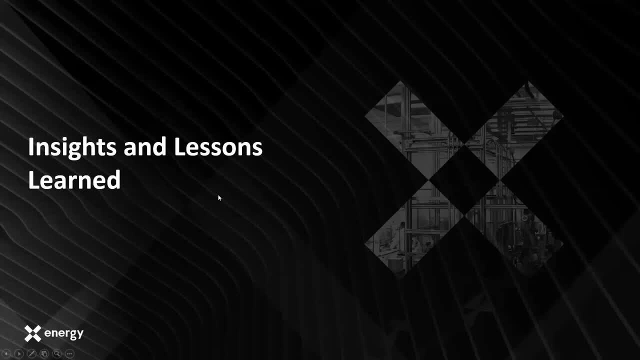 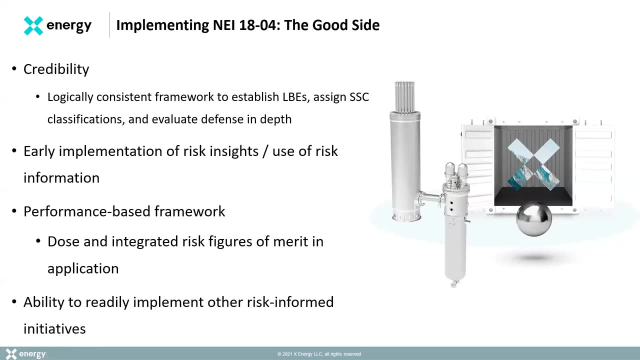 talking about some major insights and lessons learned. So one is, you know, I think all of us, you know- feel that the, you know the NEI 1804 process is a logically consistent framework to help establish the process, And so I think that's one of the things that we've learned along the 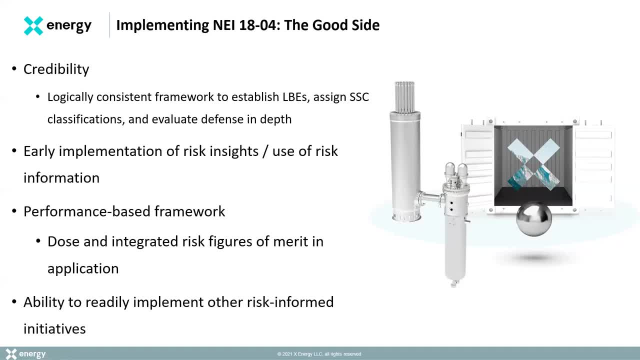 all the pieces needed to make the licensing case And one interesting story. so, as people are probably aware, you know, X Energy is involved in projects in Canada And we had one of our Canadian counterparts when they were first getting involved with this, with the project. 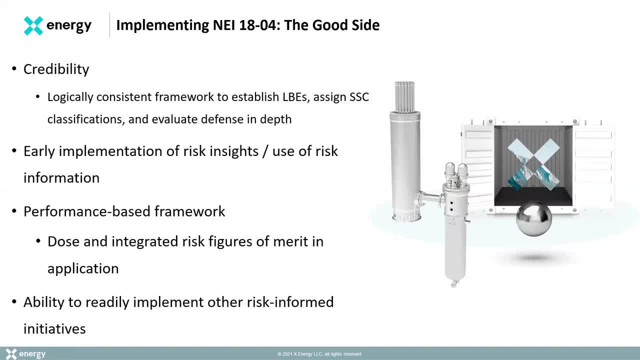 look at the NEI 1804 process, look at the Canadian process and the Canadian licensing structure. And they looked through it and said, yep, we have to do all of that And this is put together in a framework that makes complete sense. So when someone sort of from a different licensing 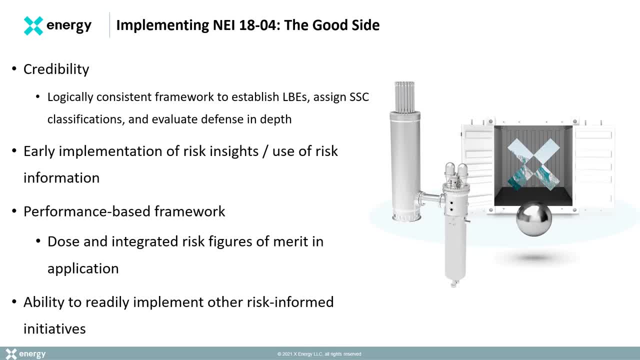 regime, you know different background, came and look at it. you know they said: you know this is something that makes a lot of sense. And even when we look at the Canadian licensing structure, you know, expect it's something that can be, you know, adapted or readily used. 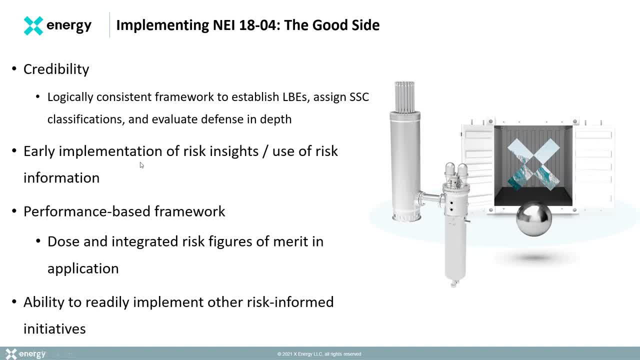 And, as I mentioned before, you know the process, especially if you, if you're building off of past designs, even leveraging, you know design insights from, from past designs helped us at the beginning, getting risk insights into the, into the, into the design evolution, And so really it's. 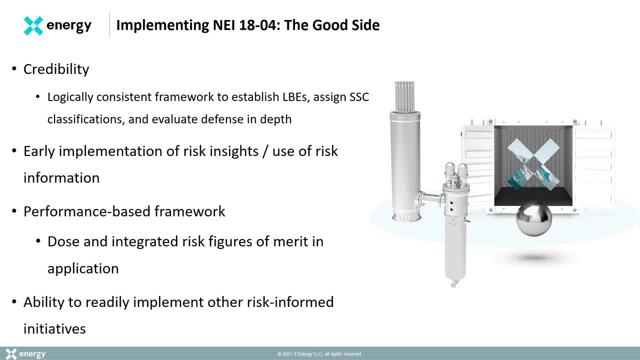 you know we can really use it along the way. You know, as long as you can maintain the consistency of the PRA with the design- you know keeping things updated- we can really use it at all various. we found we could use it at all stages and design to draw appropriate insights. 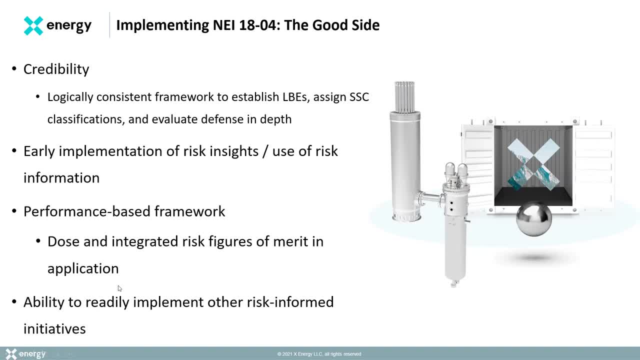 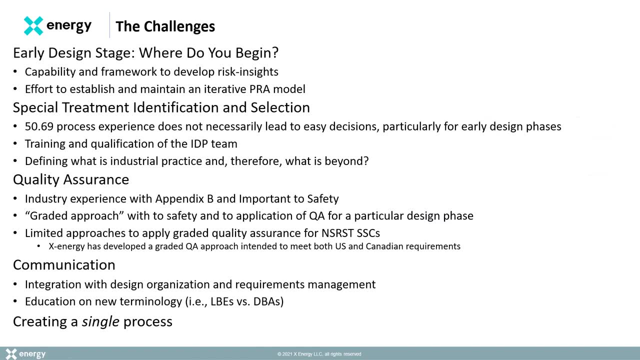 the performance based framework and it does also allow to readily implement other risk informed initiatives. So some some things that we found to be challenges. I would say that you know. you look at any. I 1804, it lays out a process and it and it talks. 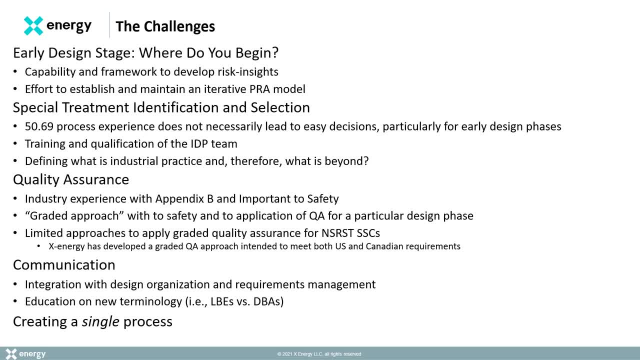 about being iterative, how one does that iterative nature. I think that's really the art, is, I think, what we've seen. So at the early design stages, you know where, where do you begin, What's the right way to start, And I and also to what's the right way. you need to integrate it with your 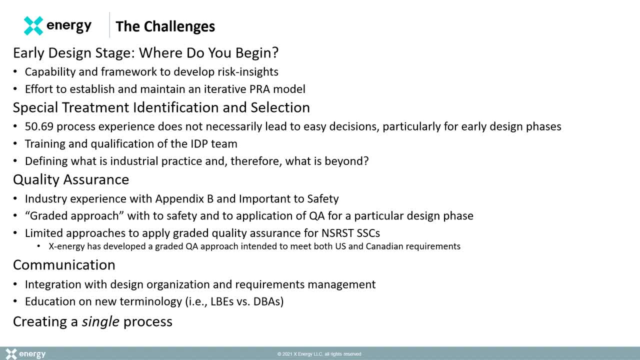 design process, Where does it involve? Where does it, Where does it fall in your systems engineering management plan? Where does it fall in requirements management? And I'll, I'll, I'll say this: I think establishing, establishing a good protocol for requirements management early on, 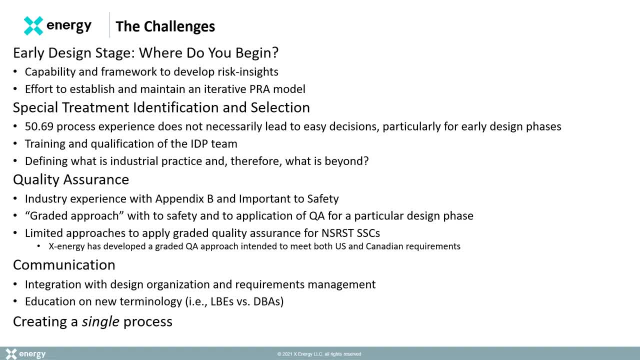 within the context of this process is really important because you have a lot of insights that are coming out of it And you know system engineers speak in the language of requirements, right? you need a good way to take the insights that are learned out of the process, you know. 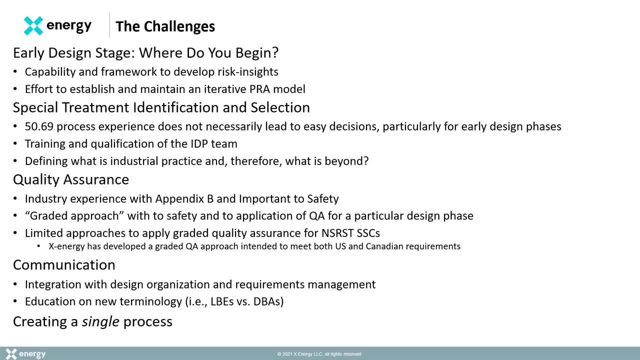 vet them and factor them into requirements so that they can get communicated and get to the right place And and get into the design. You know, and it's a challenge to to establish and maintain an iterative PRA model, you know. 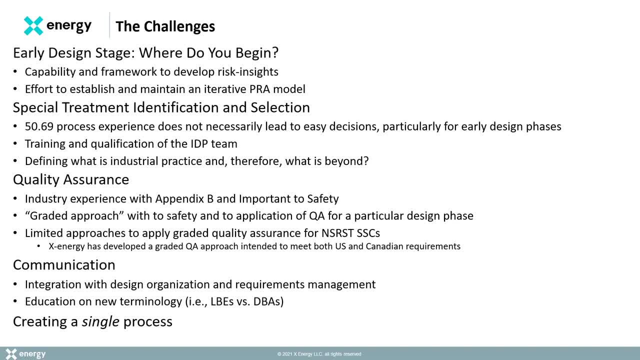 it takes a lot of, takes a lot of resources And I would say, even at the beginning, I would say it was not entirely clear. you know the level of resource that we needed, right, And I think that's a that's a challenge is predicting at the outset. you know, how many people do I need, What kind 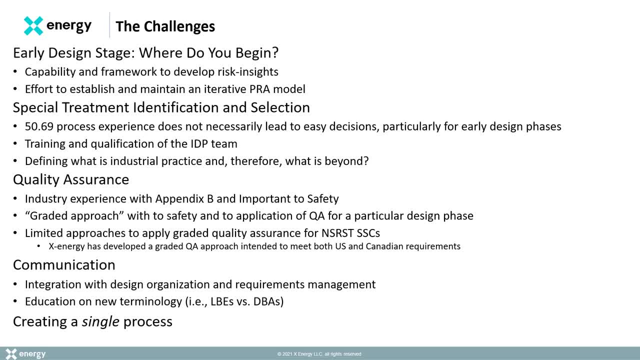 of organization do I need in order to be able to, in order to be able to implement this In special treatment selection? you know the 5069 process. you know there's a, there's a a. you know there's a lot of common with the 5069 process, but it not all of it translates. 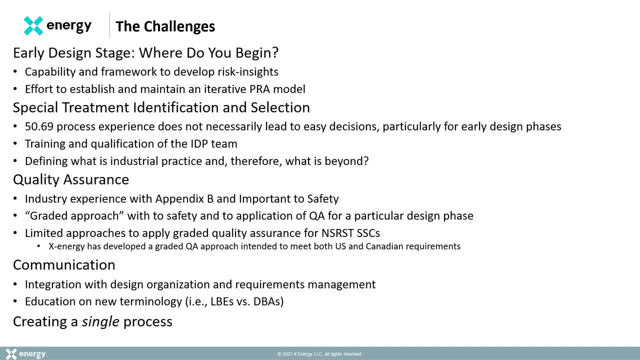 you know we've done. we've found some situations when that experience doesn't necessarily translate well because you know, bringing a lot of light water reactor mentalities over into the advanced reactor design and you have to think a little bit differently. Training and qualification of 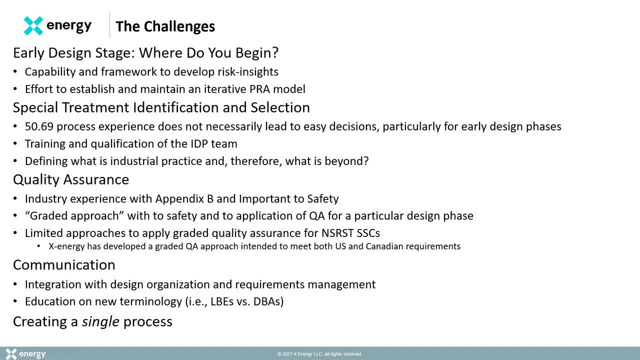 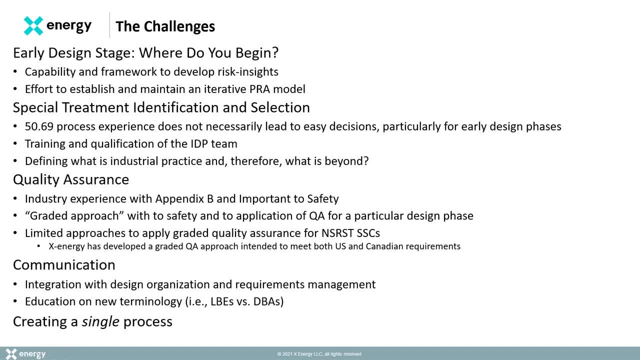 smart on this process is hard to come by right, So we need to get people trained. we need to bring more people into the fold, And usually you're having people doing double duty serving on this team. So getting the right resources in place and getting them trained is really important. 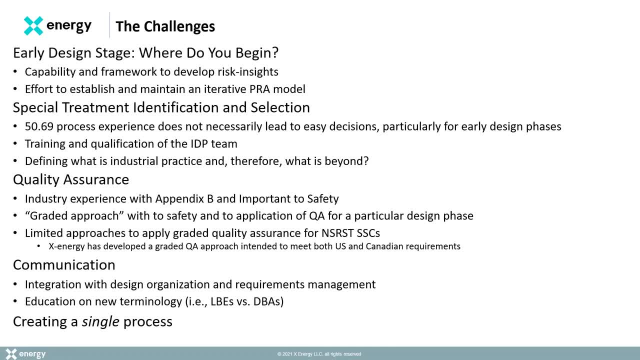 A couple different things to talk on, Kind of this last bullet, and then I get gets down into the QA section. I think are really, really important Developing a graded approach to quality assurance. You know, I think a lot of us are used to. 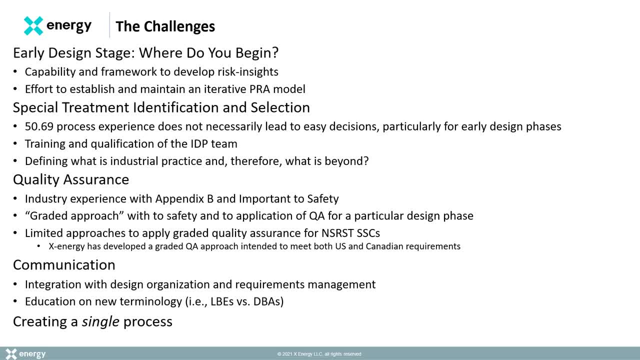 you know Appendix B and important to safety. You know there's really a new paradigm here and an opportunity to create a new paradigm and create a real good graded approach to applying quality assurance, But it's not just with respect to safety. I think one of the things we've learned 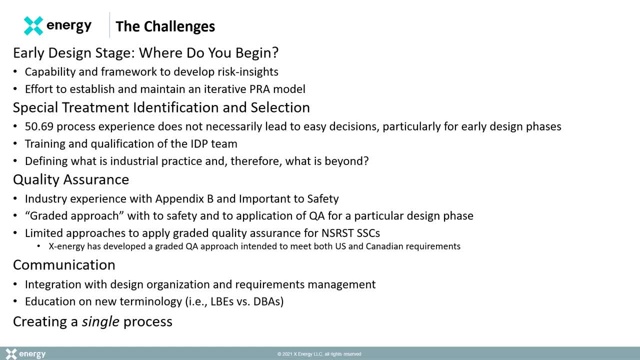 is also with respect to design phase. you have to be operating under some kind of quality management system. you know relatively early on, right, you need to have that quality management system. So you need to have that in place and there needs to be a basis for it. So you know, using the approach, 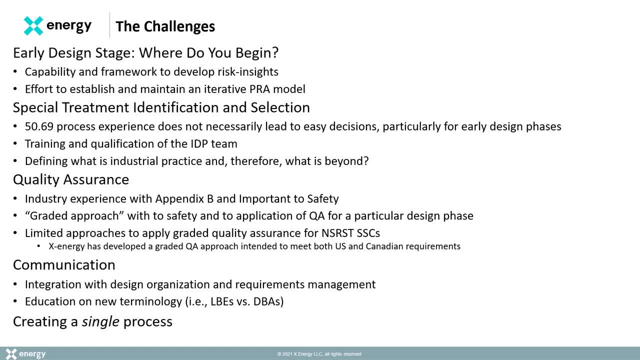 to say, to make you know incremental steps towards building the full picture of QA requirements is really, is really quite important, And one of the things I mentioned- we have, you know, working in Canada as well- is that you know, if you, if you- I don't know how familiar people are with the- 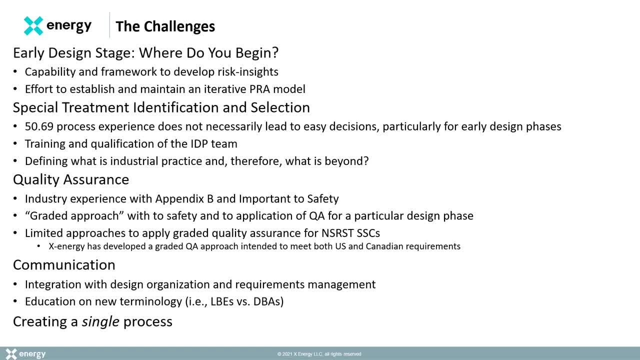 Canadian QA requirements. but you know, and what? as an American, I sort of naively went into this and thought you know, their requirements are laid out in N2C, They're the N299 standard And I sort of thought them as being the same thing as NQA1.. Well it's. 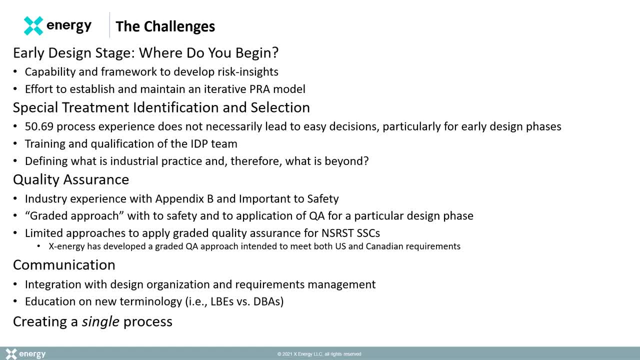 really not. N299 itself is a graded approach, And so you know that's really quite different than NQA1.. And so what we had to do is come up with an overall process to determine graded QA requirements that meet both US and Canadian expectations, And so that, I think, was a really 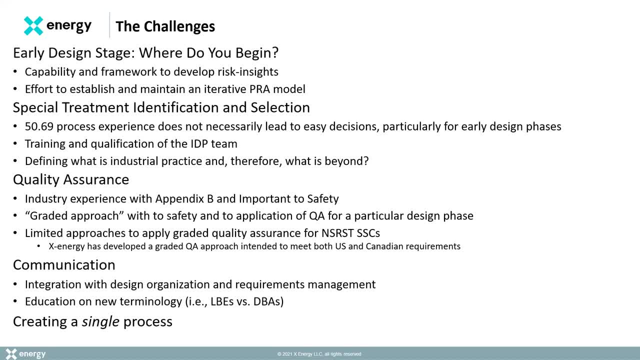 good effort And I would say we're road testing that process. So you know it's, it's great. It's not only with respect to importance to safety, but also allows us to phase it as a function of design so that the design teams can operate. You know they have justification. 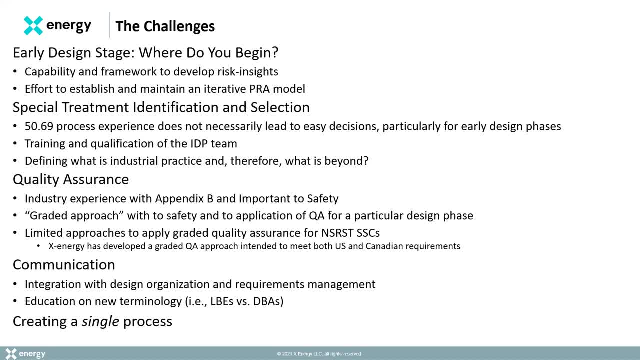 for operating under a particular QA program all throughout the design process and allows us to refine it along the way. Just a couple of final things to touch on. I mentioned this a little bit: communication, you know, integration with the design organization and really having a good 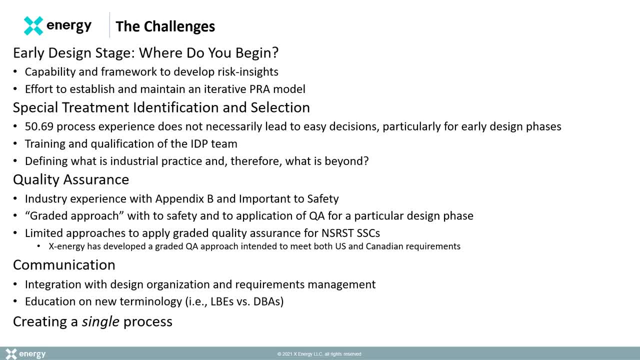 way of communicating requirements, Because, again, we generate a lot of insight. You have the ability to do a lot of things, And so, you know, I think that's a really good thing, And I think that's a really good thing to do, And so, you know, I think that's a really good thing to do. 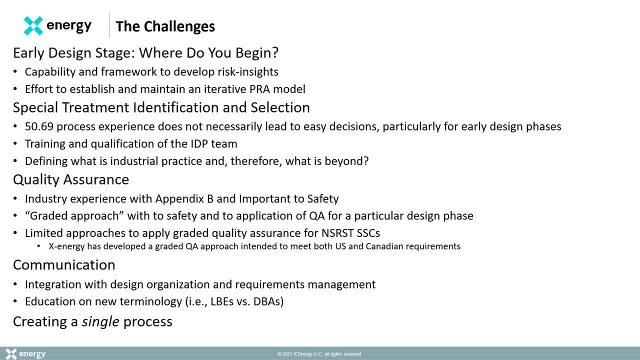 And education on new terminology. Like I said, the number of times I've had to explain DBEs versus DBAs, well, I lost count, you know, nine months ago. So that's an important thing to be able to try to get. 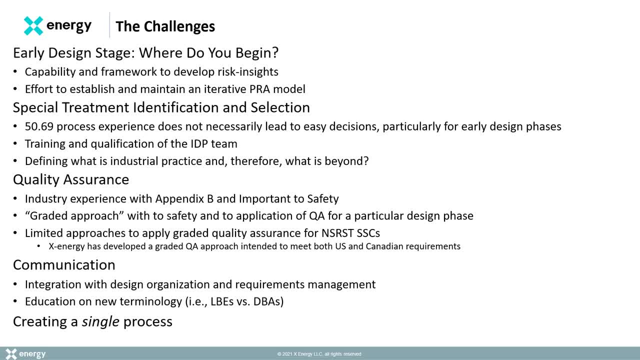 that terminology, get people understanding it, And then finally, as I mentioned, creating a single process, right? So I see NEI 1804 as a set of tools And, you know, an organization is going to create their own process depending upon what's important to them. 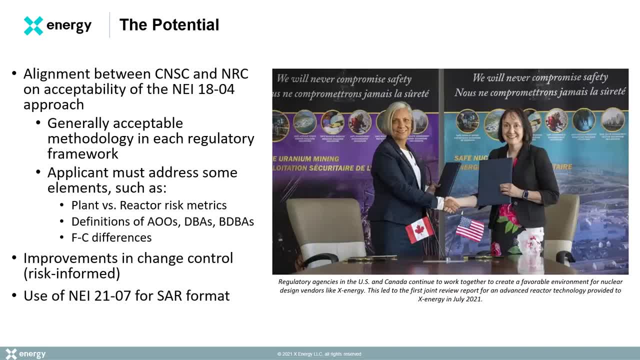 And just a final on the last slide here, final, some few concluding remarks. You know, again I mentioned the engagement in Canada and I think we've seen a lot of positive movements And I think there have been some. I think there was something recently issued by the NRC and the 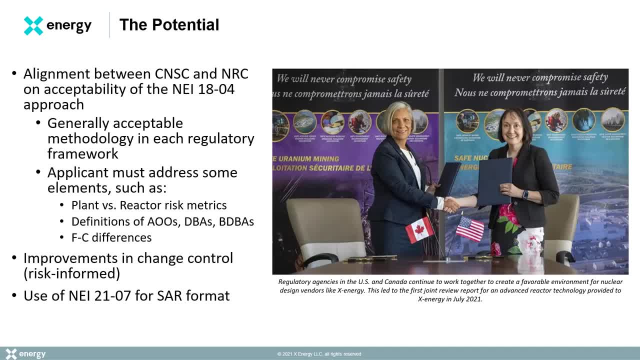 CNSC regarding, you know, generally finding NEI 1804 acceptable. you know it's not an endorsement, But I think across our engagements there we found that the NEI 1804 process has a lot of traction And so, really, 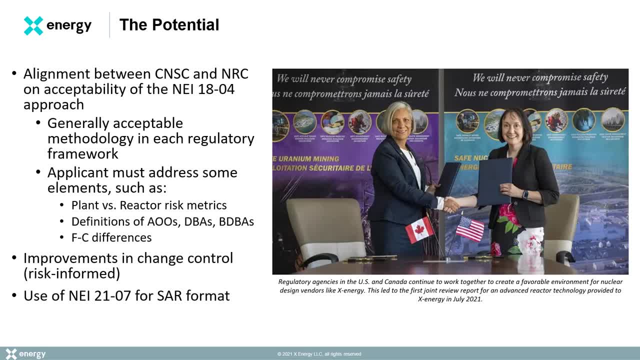 a great potential there and being able to apply it across regulatory markets. And then also just in one thing to close off on is the use of NEI 2107 for a SAR format. So that's something we haven't committed to, but we're actively looking into it since its release. 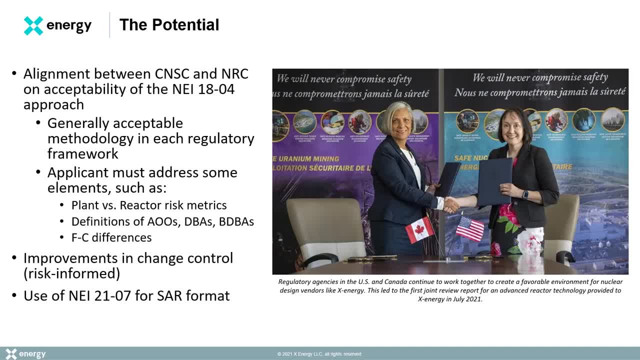 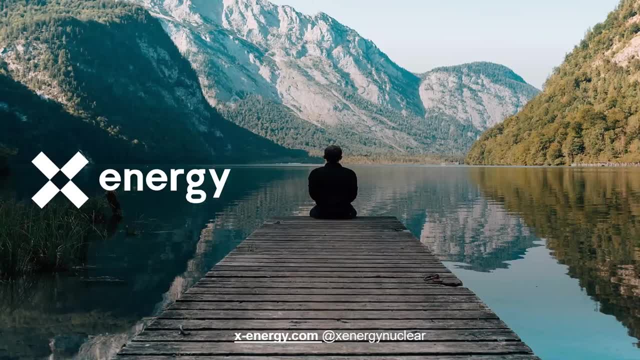 with the preparation of our own SARs. So with that, I thank you for your time and attention And I will take any questions that you may have. Okay, there's a question on the chat from Bob Martin. Yes, Can you read that, Kyle, or shall I? 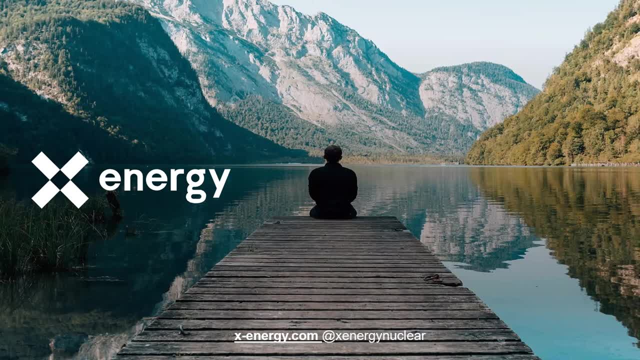 Yes, I got it. So you stated that you only considered internal events. What have you done to address external events? So I'll say that first. So we have since started to incorporate external events in the PRA. that was noted at the time. External events were not. 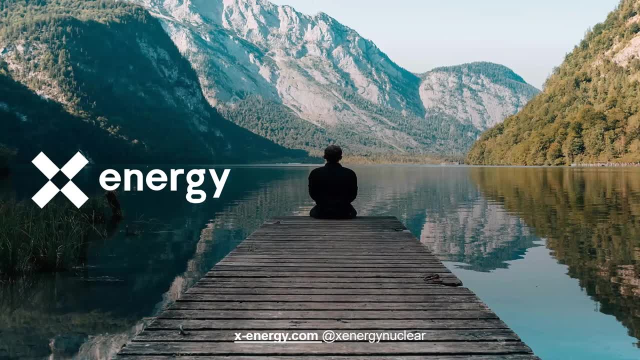 included, although I'd say we've been implicitly including them, at least in our thought process all along the way, because we know we're going to have to, even though it hasn't formally gotten into all aspects of the PRA yet. On the second item, for mechanistic 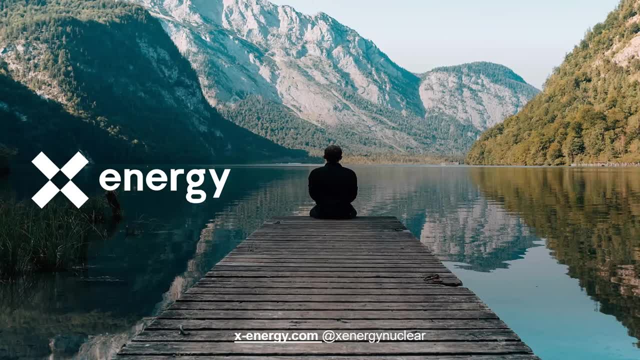 source term calculations. did you use off-the-shelf codes? You develop it from scratch, And so that was the excess term code that I mentioned was an in-house developed code. Okay, I don't see any other questions in the chat, but I had a question, Kyle, on slide 14.. If you, 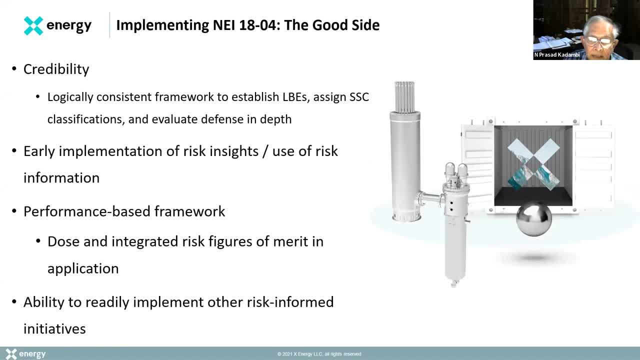 go to that. yeah there, This idea of using figures of merit as a means by which you can set decision-making criteria right. That's how you use it. You say that you use a dose and integrated risk, but how about, you know? you said a key part of this whole thing is margin management. How about? 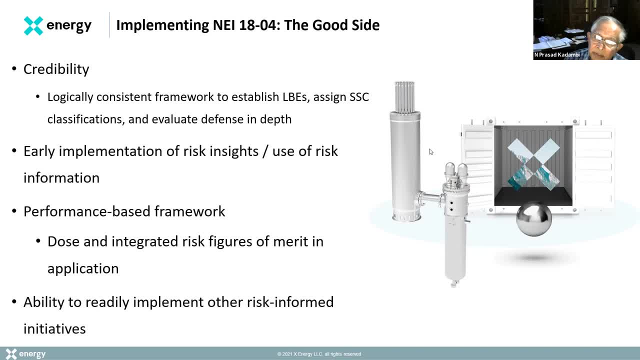 figures of merit associated with margins at different levels in the hierarchy of the requirements. Have you thought about that? I would say we've not formally. I mean, I think that we've had conversations about margin management but, I would say, have not yet incorporated that into our thinking as of yet. Most of 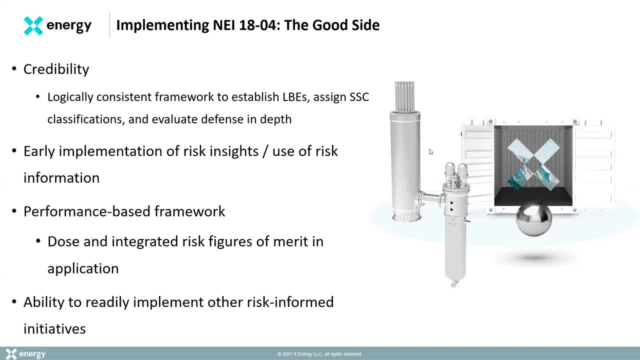 what we've been looking at in some of these figures of merit have to do with how we set importance relative to establishing QA requirements. That's kind of what we've been focusing on so far. The margin management discussions, I would say, are ongoing. 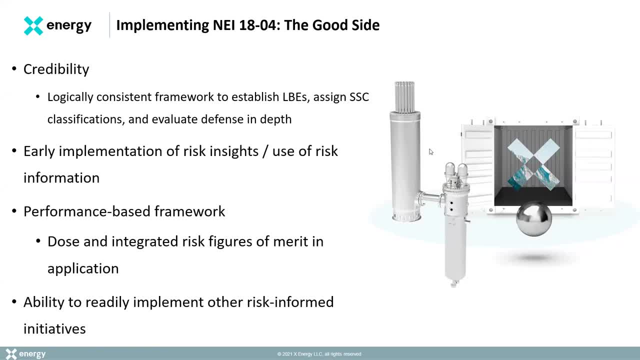 but we haven't made decisions yet with regards to how that's going to be explicitly incorporated. Let's see. There have been a couple of other questions. Perhaps you can pick up on them. Yes, Because they're coming rather fast right now. 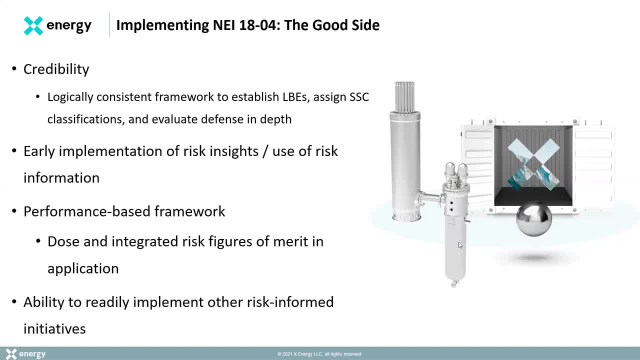 So when I let me look at so. first question from all right, so thank you for the presentation. I do have two questions. What was your screening criteria and how do you handle uncertainty? So I'll address the second first, because I may need to ask you to do a follow-up on exactly what you mean on the first one. 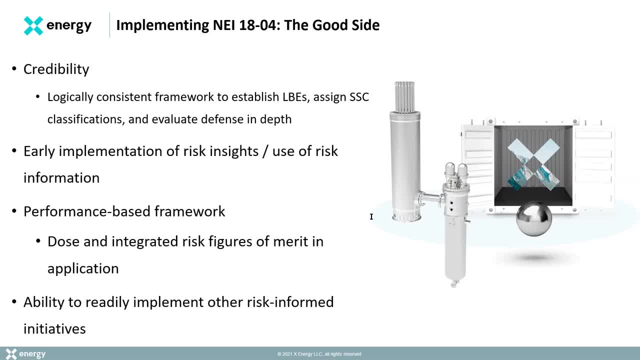 And so handling uncertainty right now. So in the initial PRA, you know, there was no explicit treatment of uncertainty. But we are work, we've developed uncertainty, we are developed and developing uncertainty quantification methods to be incorporated into the FC chart as we speak. So that's, that's ongoing. And on the screening criteria, is what is your? I can interpret that a couple different ways. What's? what is your exact meaning there? 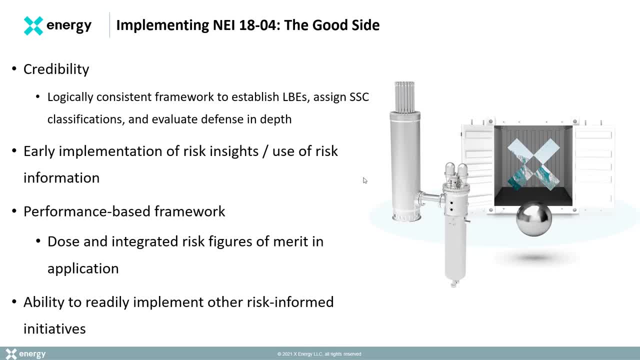 But perhaps the person can go off of the chat and off of mute and you can state your question if you wish For sure, Hello, Yes, My name is Agyeman. I mean for the screening criteria. you, we have many internal events or initiating events. you pick some of them. 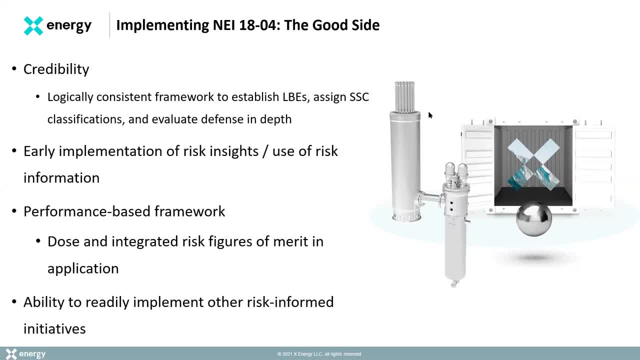 I think you have some screening criteria to not to include other initiating events. Sure, That's what I mean. Yeah, Sir, I understand. So I probably can't give the best answer to that. The PRA folks working could probably do better than me. 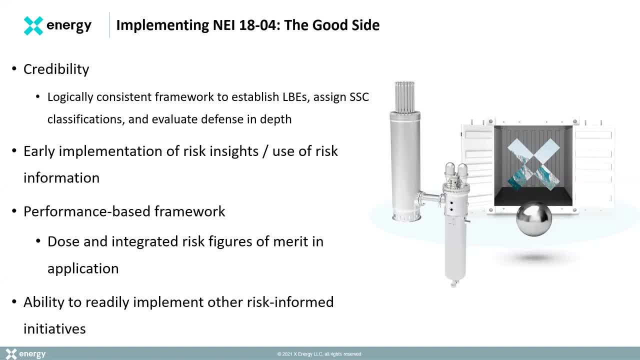 All what I'll say is that you know we're using the ASME non-lightwater reactor PRA standard And my understanding of that standard is that it has a methodology in there for screening, internal screening, what events you have to consider, and we're following that process. 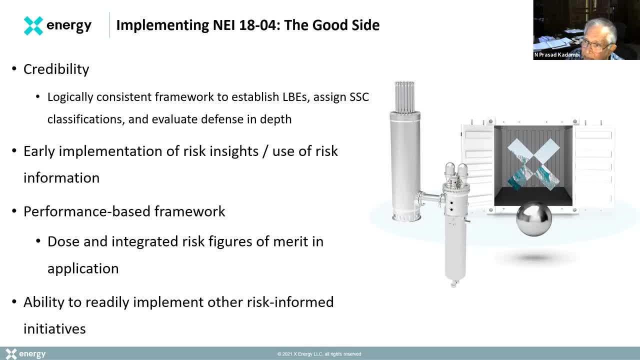 Thank you. Thank you, Let's see. There are a couple of other questions. One from Eric Osterly: Yes, So in the column on dose you indicated M or P for various event sequences. Oh, so that's kind of a holdover from that old phase zero PRA, because it's, it's, it's when it was originally. 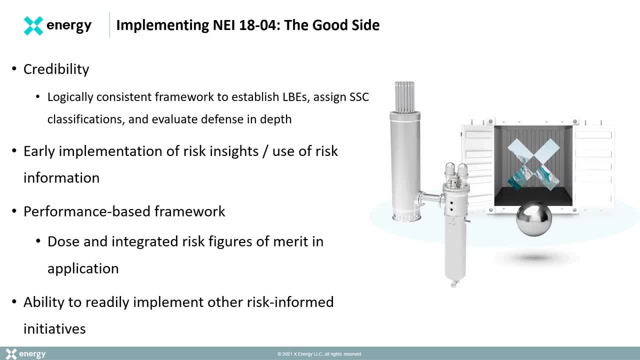 when the doses were originally developed, both- I think it was the MHTGR and and PBMR were used as as the dose, as the source of the dose information. So it was. it was indicating whether or not it was a the MHTGR, I believe, or the PBMR source terms, where that was based upon. 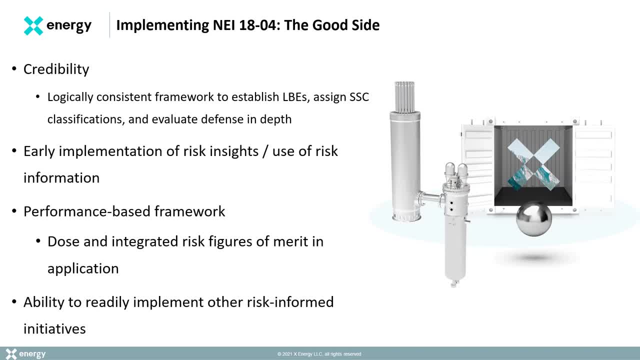 But it was. it was basically the source of the dose information that was used. Next, Andrew Clark, for the PRA model: Are you relying strictly on absolute risk metrics or are you leveraging some relative risk metrics? We're using both And you know, in different, in different circumstances, but both yes. 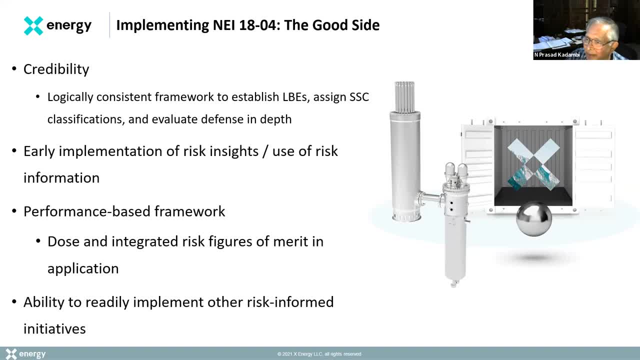 Then, Mark Joseph, perhaps you can read it. Sure, yeah, I'll take care of it. Yeah, So question on use of 1E-4 limit for design basis compared to use of 1E-6 as limit for for DOE reactors is: is the use of 1E-4 based on a standard or expected to be accepted by the NRC? 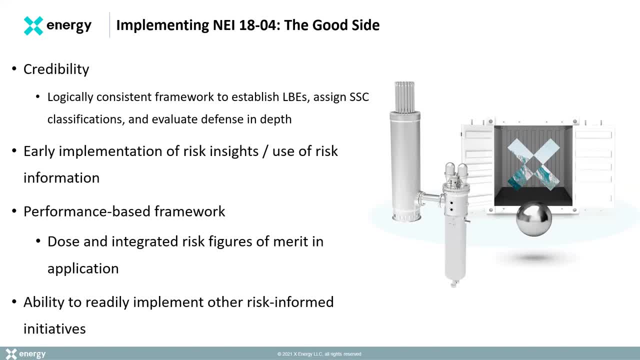 So you know the 1E-4 for DBEs. you know this. this was what was laid out in NEI 1804, and my understanding endorsed as part of Red Guide 1.233.. So that's my understanding is that that those categorizations have been accepted by the NRC. 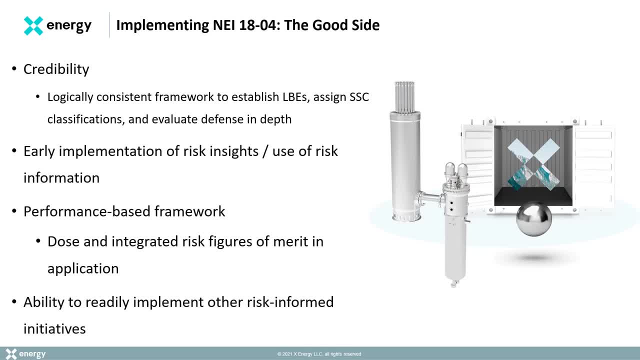 Yeah, I don't know if you want to discuss that anymore, but it it seems like a pretty significant change. I'm just not familiar with the use of 1E-4 versus 6.. I mean, I agree with the minus four because you know there's certain design. 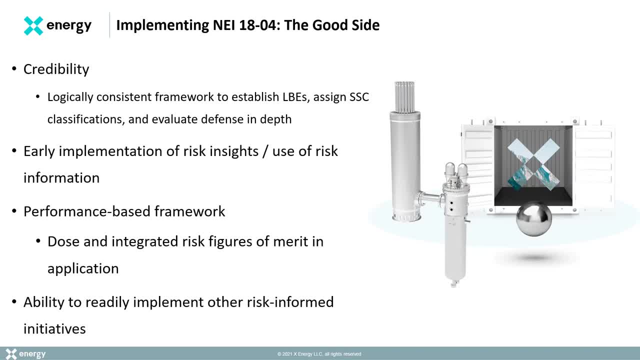 there's certain design basis events based on either minus four. However, beyond, design basis is pretty much, you know, either minus six. Yeah, I will admit that I cannot comment very well on that because I mean I would speak to those who may have been involved in the. 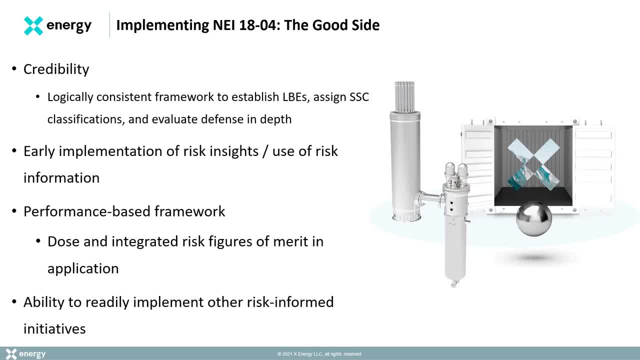 in the process in developing NEI 1804.. I can't comment on on what the basis behind that was, unfortunately Okay. So there's the next question from Bob Martin. Perhaps you can address that. Yep, So a key challenge for applying NEI 1804 to a first-of-a-kind design. 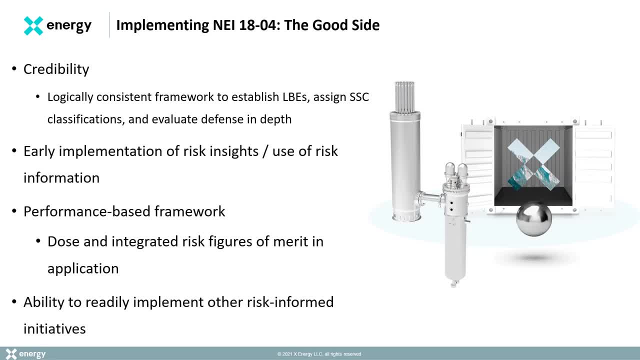 there's no design-specific operating experience. to draw frequency and reliability data from using the limited data from the few HTGRs that have been built and operating would seem to be very out of date, Although an argument could be made that data would be conservative. 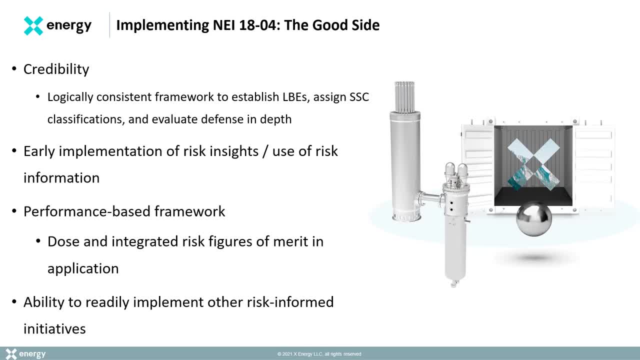 How have you gone about justifying the data you used to populate the PRA models? No, it's a great question And actually it was a sentiment that I wanted to touch on, but didn't You know? I think you know we use the data, the best available data that we have. 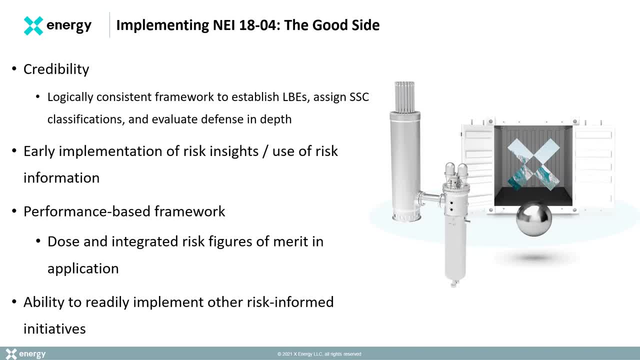 You know some of that comes from you know available sources in the industry now And some of it might come from you know- I don't honestly know what data the PRA team is using that might come from you know the past HTGRs. 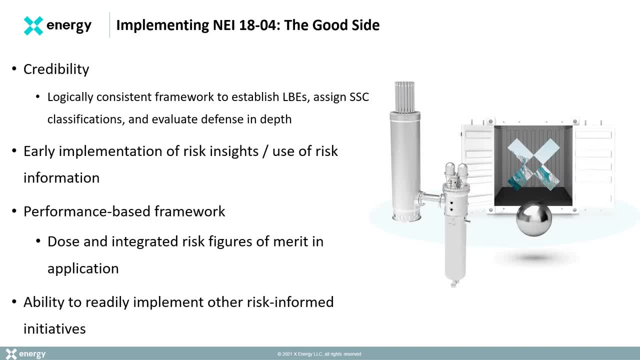 But you know, essentially we have to recognize that there's uncertainty and try to make decisions commensurate with that uncertainty. And so I would say, you know, we use the best information that we have, try to understand what the key importance drivers are and understand you know. 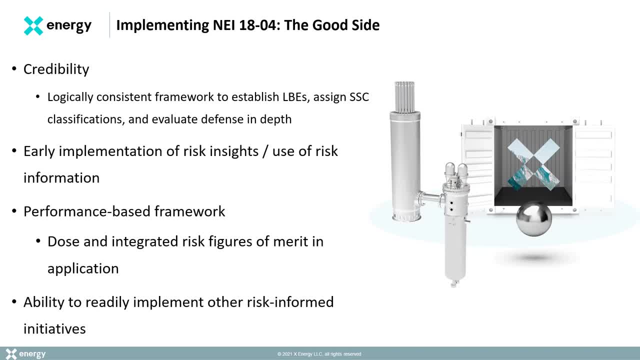 if, if there's uncertainty, If that thing is important, but it's it's using using values that we think have a lot of uncertainty associated with it, then we have to adjust our decision making appropriately. That's a very probably confusing answer because it's it's very situation specific. 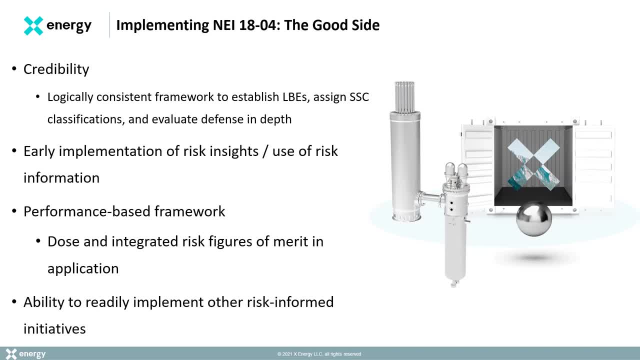 But I think it's the idea of looking at: okay, I need to make a decision right, What information is available to make that decision And how confident am I in it, And we sort of make that judgment as those things come up. 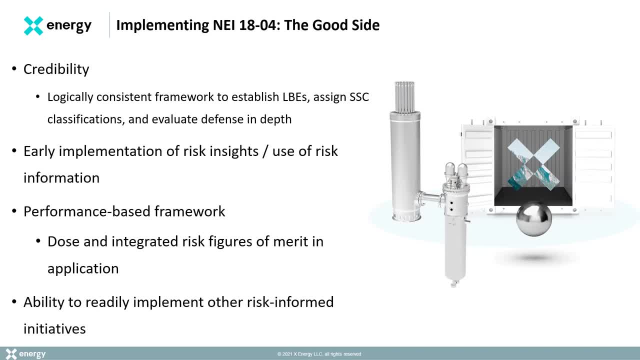 And if we find that there's not a lot of basis, that there's not a lot of evidence behind the numbers that we're using in a certain circumstance, then we either have to take an action to go get more information, or you know, you know. 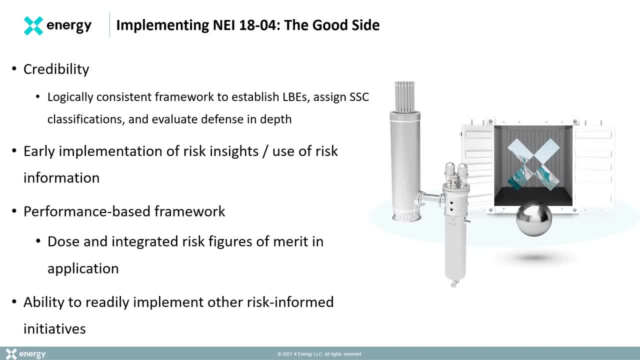 or, or you know, build in margin or something right. So it's it's. it's hard for me to answer generically because it's a very situation specific thing. So next question from Jared Valeri: physical security scenarios. 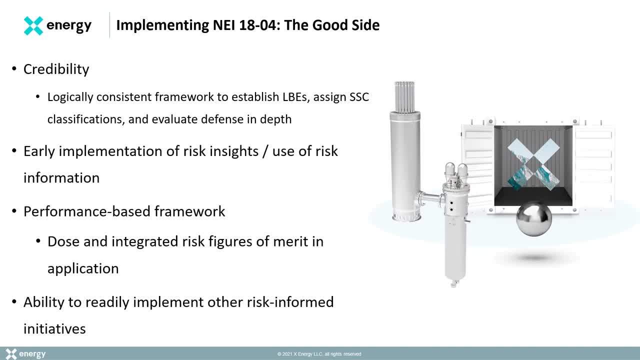 At present. no, They have physical security scenarios. Physical security scenarios have not been, have not been yet can get considered. See, and I think there is a comment from Bob Martin that the 1e-4 comes from a DOE document. 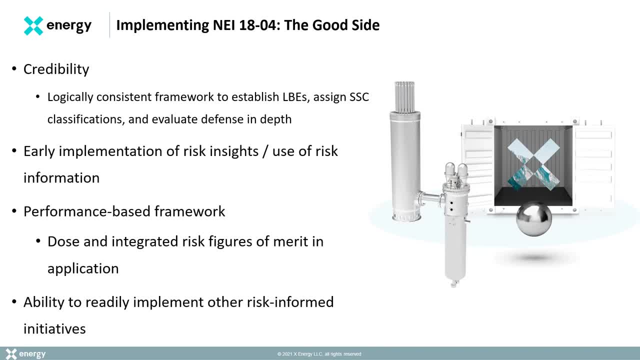 Yes, the 1e-4 comes from DOE handbook 1224,, I believe, is what Bob says. Okay, that's great, So okay. one more question. I guess we still have five minutes, So Go ahead. 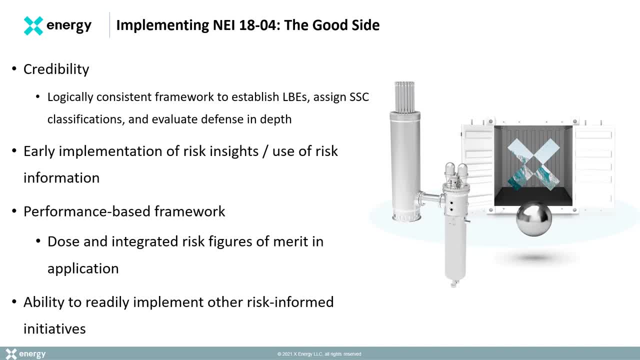 Yeah, so NEI 1804 has three categories for LBEs: AOOs design basis. Yeah, I think it's looks like it's a follow on to the comments of the AOOs design basis. events are greater. 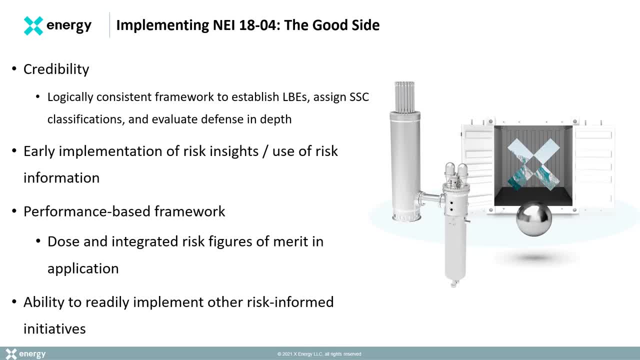 than 1e-4 and beyond design basis events. that goes from 1e-4 to 1e-7.. All three are considered in the LMP process. Great Thank you for clarifying, Mustafa. Okay, that's great. 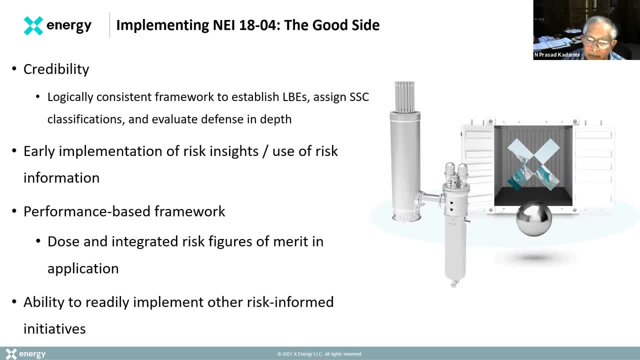 Kyle, you handled quite a number of questions. If people have any more questions and you're able, to enter it into the chat before we close off, We do try to limit this community of practice session to one hour because we find that's what people plan for. 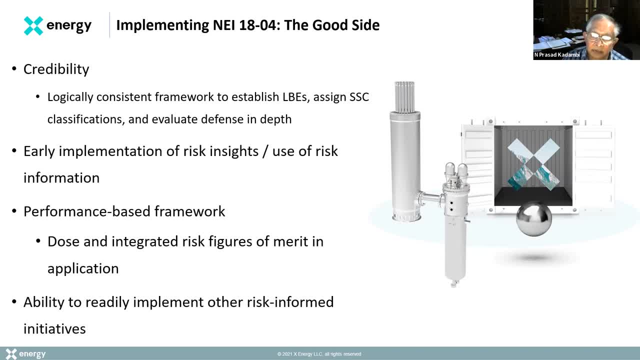 Okay, Thank you for clarifying, and we don't want to impose on their time more than they plan for. But again, Kyle, I want to thank you very much, you know, for coming forward and making this presentation. I think it has.